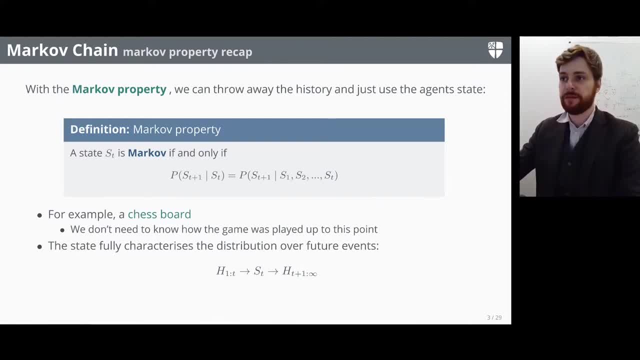 property was, or what Markov states were, information states as we also called them. So here, if you remember, a Markov state was just one that completely sufficiently captures all future events, So you can throw away everything before it, if your dynamics, if your environment. 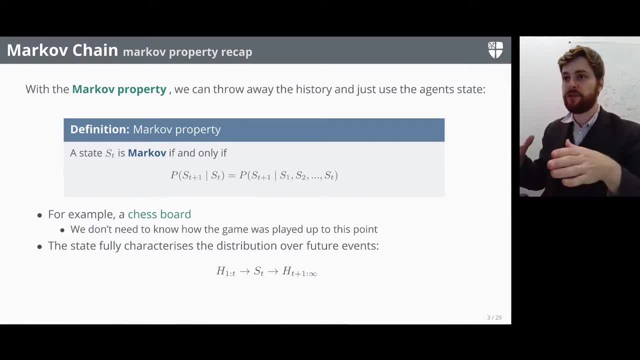 can be expressed in terms of Markov states. For example, if you have a chess board, just by looking at the chess board you actually know everything you need to know about the game to be able to behave optimally from there on. You don't need to know up to that point in time how, what moves your opponent played or 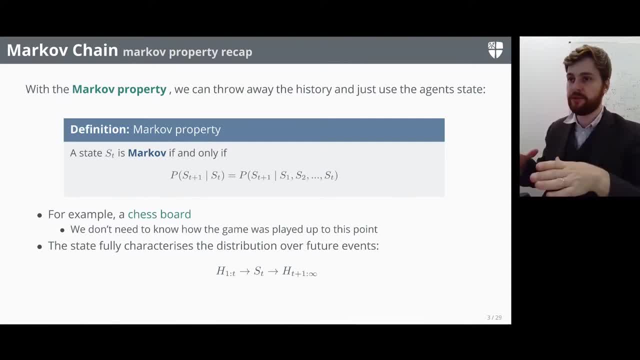 what moves you played sufficiently. by looking at the chess board, you know how to behave optimally from there on. And if you remember, conversely, we talked about that example where there were cars in a race and if imagine, there were two cars close to the finishing line- 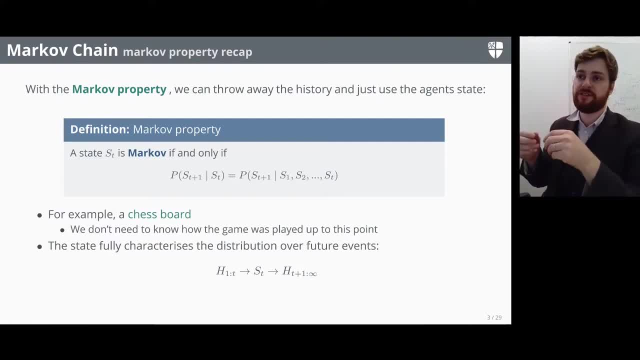 if you just look at the chess board, you know how to behave optimally from there on. If you just had their two positions, that wouldn't be sufficient to tell you who is going to win the race because, for example, one of the cars might have broken down, the other car might be accelerating. 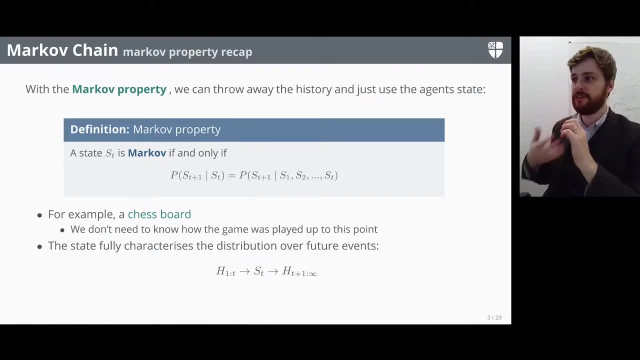 rapidly. You really need that extra information. you need the velocity, the friction, the weather conditions, the car weights. you need all of that to be in the states themselves, to make them Markov, to be able to make them sufficient to tell you who's actually going to win the race. 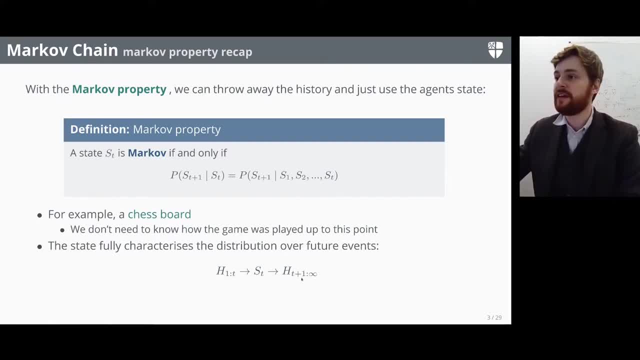 Then we had this equation down here, or this notation, where we said: the distribution over the actions and events of for the entire future is conditional only on the Markov states, which is the same as if it were conditional on the whole of history. So you can actually throw away all. 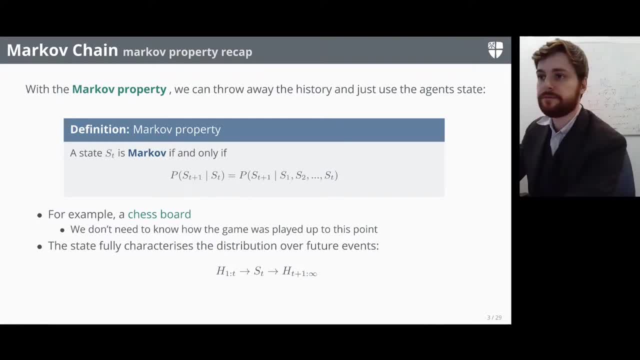 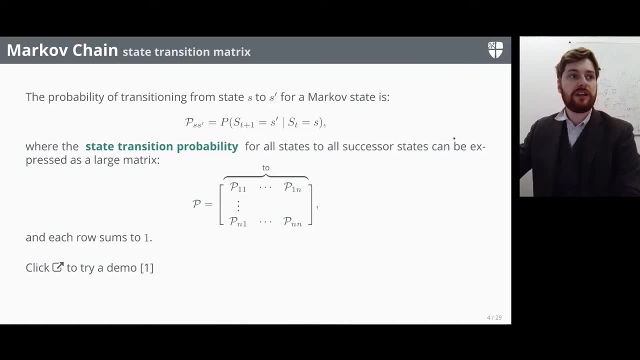 of history if your states are Markov. So what is a Markov chain? Well, simply, a Markov chain is where you've got your states, like being in the pub, being in your room, being in the car. So you've got these kind of labels for your states. So you've got these kind of labels for your states. 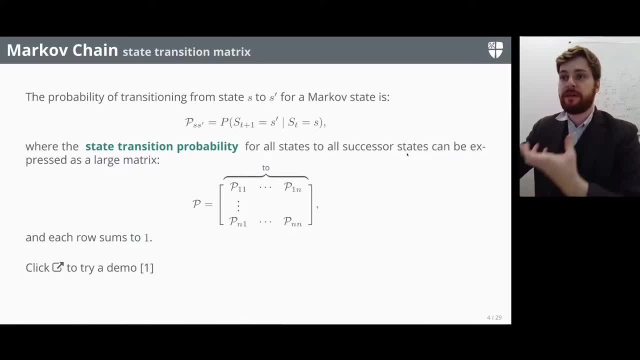 So you've got these kind of labels for your states, But you also have the dynamics. you have the probability of transitioning between the states. So you can express this as a state transition matrix, or this is how we would define it. We would say there's some probability of going from 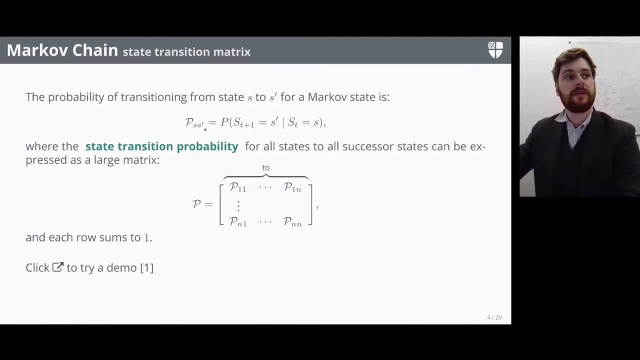 one state to the next state. this s prime, and that's just the probability of the next state, is conditional on the previous state, So this is some probability of transitioning from state to some other state, And for all the states in our environment we would represent these. 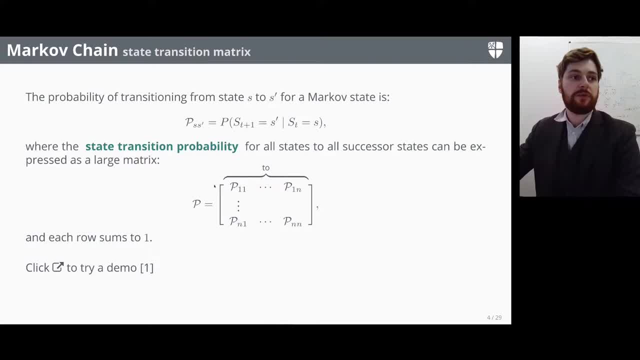 probabilities as a matrix where you would have down here you would have like a, b, c and the probability of transitioning to the states a, b, c here. So I could give a sort of very simple example just in my notes here, If I just push this down. 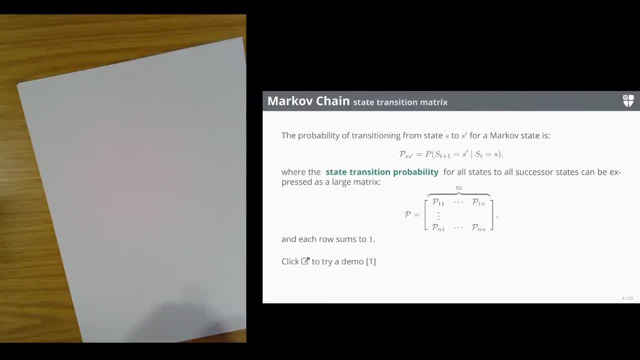 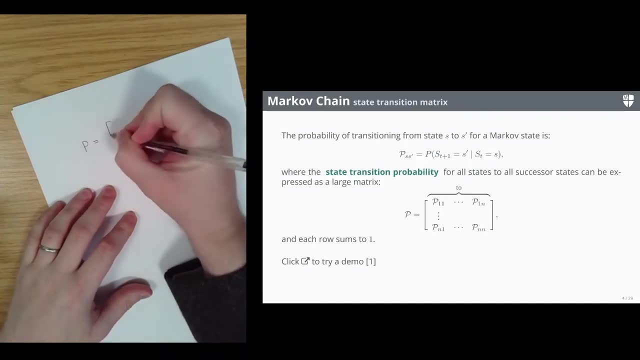 I'm just going to switch that over. So a very simple example of a state transition matrix would be to say: p equals. maybe we've got some state a, b, c. We could just say, for example, there's a 0.3 percent probability of the state a transitioning. 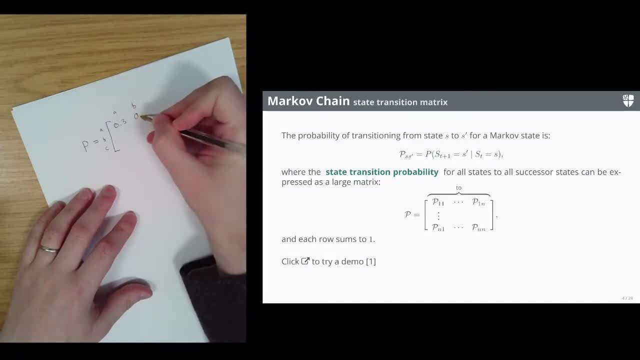 to itself. then there's like a higher probability of transitioning to the next state b, then there's a lower probability of transitioning to the next state c And b could be, for example, a 100 percent probability. it always transitions to state c And state c. we could say: 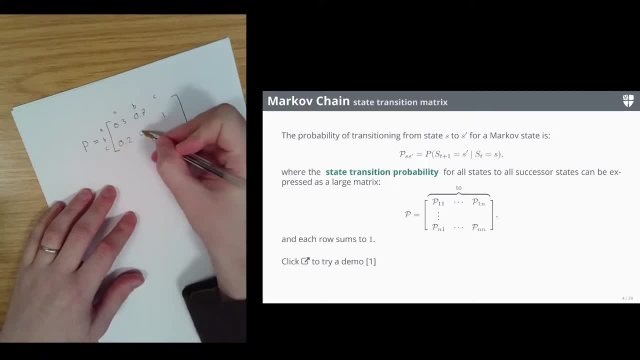 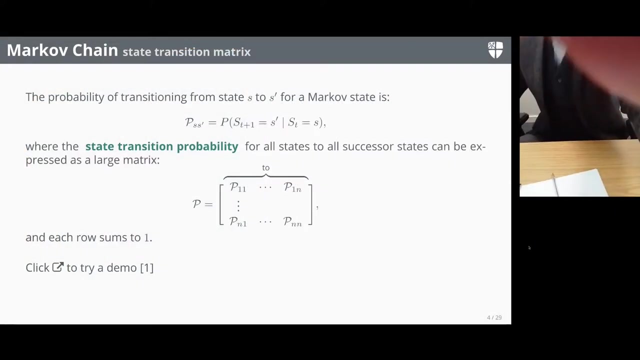 has a quite low probability of transitioning to state a, quite a reasonable probability of transitioning to state b and also quite a reasonable probability of transitioning to state c. So that's an example of a straight state transition matrix. Okay, Just bring that back. 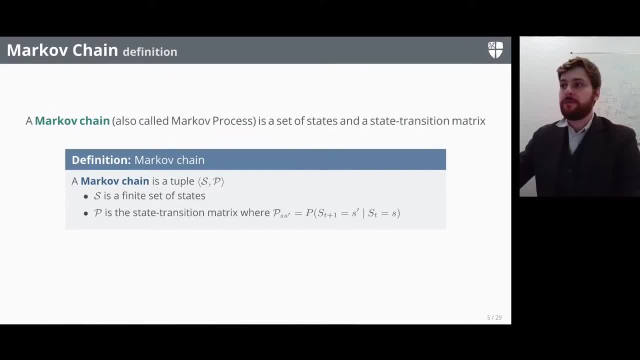 So we've also already sort of briefly touched on what a Markov chain is. but a Markov chain, also called a Markov process, is simply the labels of your states, or a set of states, and also these transitional probabilities, this matrix here, if you like. So formally it's a. 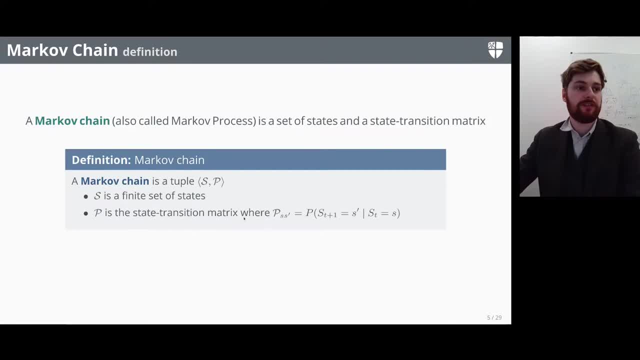 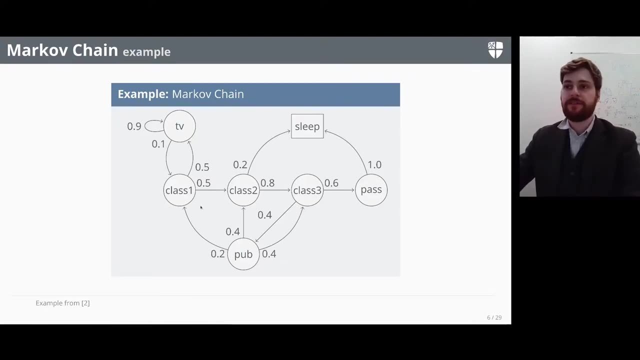 finite set of states, where p is the state transition matrix and we've already looked at that equation, The probability Which captures the probability of transitioning between the states. So this is a really great example by David Silver and it really sort of shows a nice 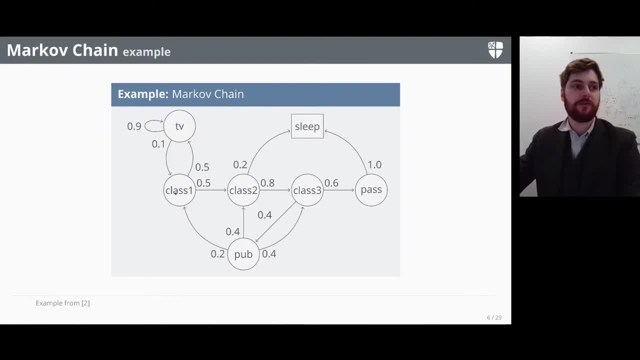 concrete example of a Markov chain. So I'll just walk through this. Basically, we have these states, We have the state of being in one of the classes, maybe on this course. So there's three classes you can attend And if you go to all three classes then you could. 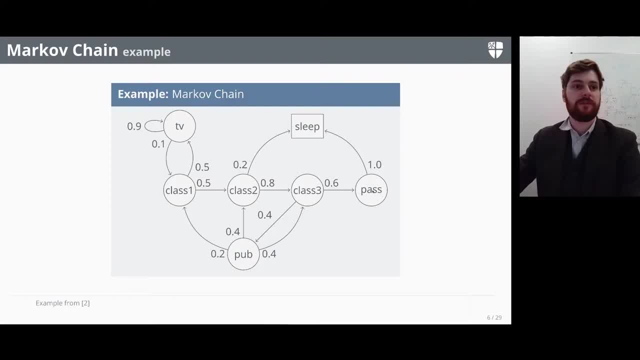 hopefully pass. And then, once you've passed, with 100% probability you can go to sleep and you're done. But also, if you're in class one, you might find the content slightly boring, So you might decide to watch TV. There's an equal probability. you could go to transition to class two. 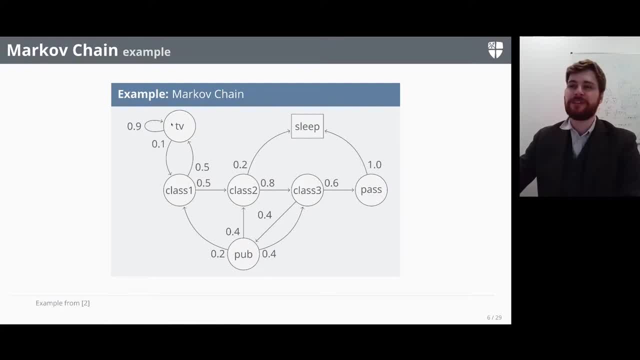 but equally, you could transition to watching TV, But when you're watching TV- maybe your favorite TV drama on Netflix, let's face it, there's a very high probability you're just going to keep watching TV, So you're going to be addicted to Netflix. 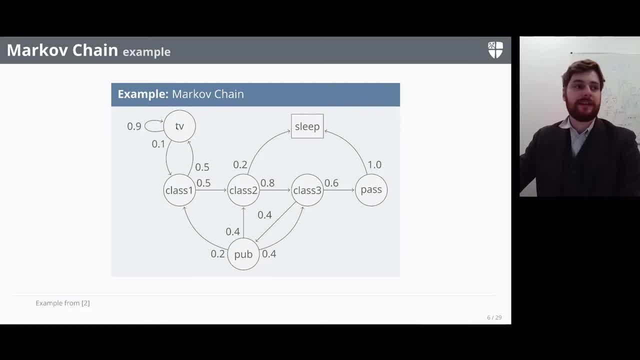 And there's a very low probability that you're going to actually come out of that state which transitions to itself back into class one again, And when you're in class one, hopefully this time you'll transition into class two, And maybe now, with a high probability, 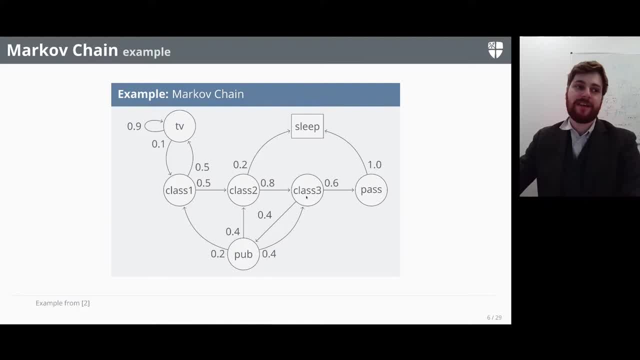 you'll go to class three. But now you're in class three, you might be quite tired, so you might decide to go to the pub, with some probability 0.4.. And when you're in the pub, who knows where you're going to end up? I mean you could. 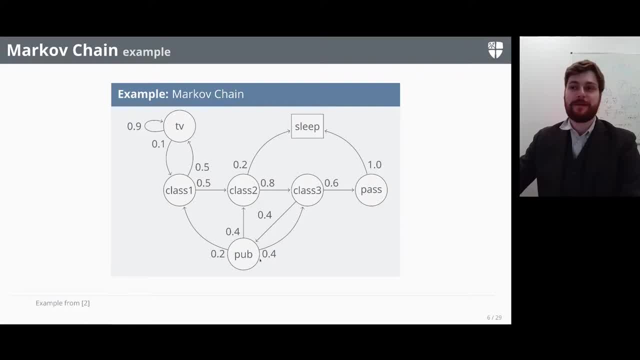 end up going back to class three, But maybe you've had one too many drinks and you need to remember what you just studied So you might go back to class two. Or maybe you've really had too many drinks and you're gonna have to go all the way back to class one, because that's basically. 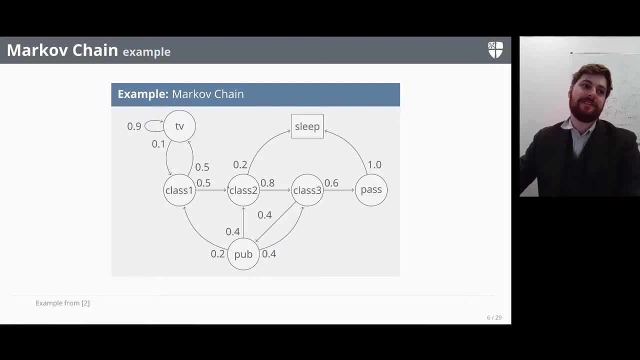 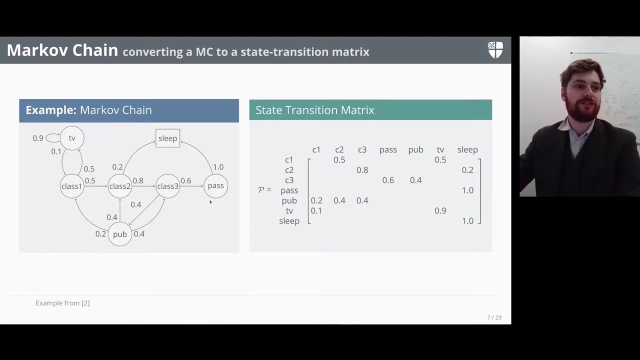 you've just forgotten everything. Then when you're in class one, maybe now you transition back to class two again, But maybe now you've had enough, so you just go straight to sleep. So we can actually represent that whole process as a state transition matrix, all of those dynamics where you can see the states. 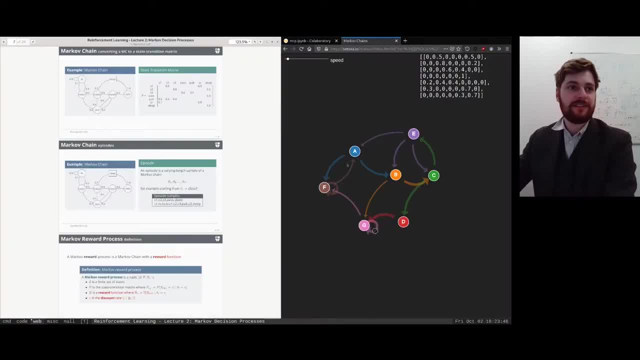 captured here and here, And actually there's a nice demo And I've just sort of plugged in something similar to that here So you can have a look at how the agent interacts. Currently it's stuck in one of these self-transitioning states And now it's here it is, it's playing. 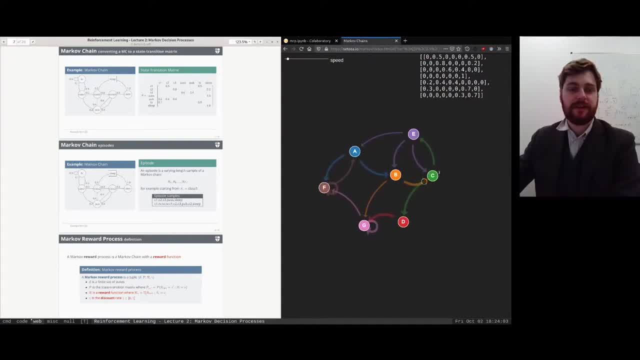 an episode And you can see how it transitions around the states And you can see how it's with some probability here it's stuck in this self-transitioning state g- again, Maybe that's watching TV, and so on. I've just removed the terminating state here. 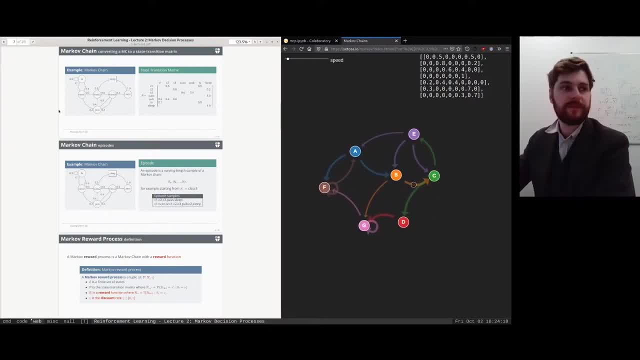 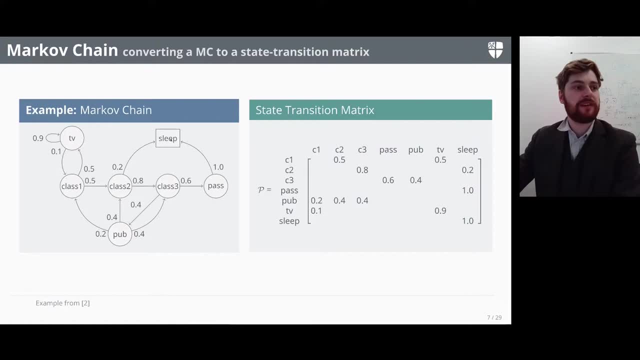 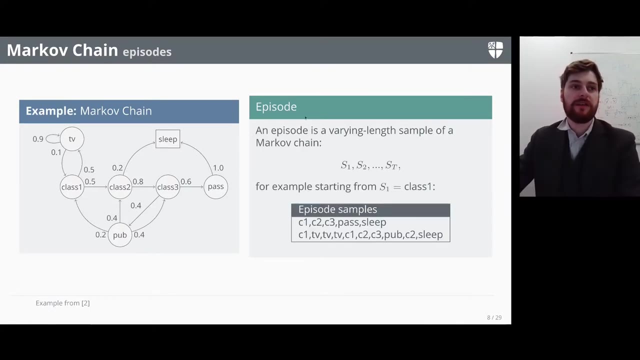 Otherwise it would get stuck and be a bit boring. So once you finish and you reach a terminal state, we would say you've completed the episode and you're done So formally. an episode is a varying length sample Markov chain, So it's where you go through you start. maybe we start at class one always. 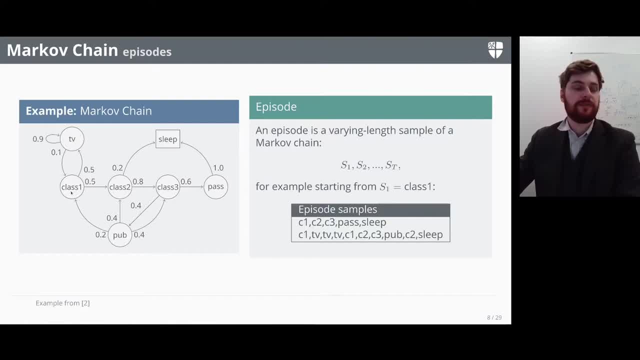 maybe that's our initial state and then a short episode might be- or an optimal episode might be- to transition to class two, then on into class three, then pass and then you're done, you can go to sleep. So that's quite a short episode. An even shorter one might be to go from class one. 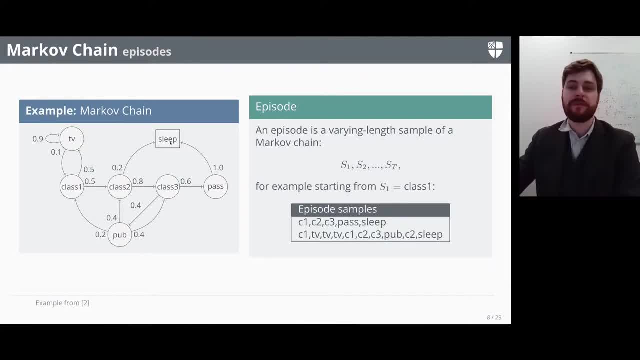 to class two and then straight away to sleeping. But similarly we could have a much longer episode which is where we just sample this Markov chain and we start in class one. then we start watching Netflix on TV. we keep watching another episode and then another episode, then we go back to class. 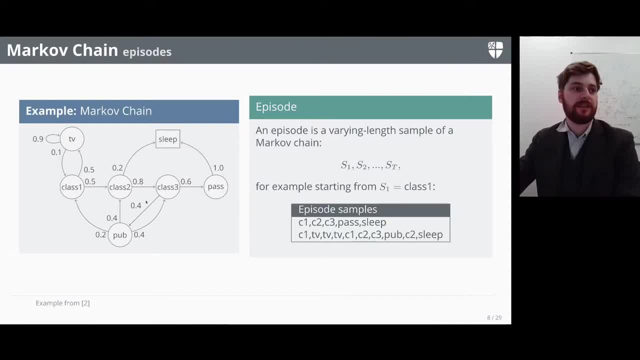 one, then we go to class two, then we go to class three, then we go to the pub again, then we go back to class two and then maybe you sleep. So these episodes can actually be very, very long, but because of the Markov property you're always going to terminate eventually, so it will always be. 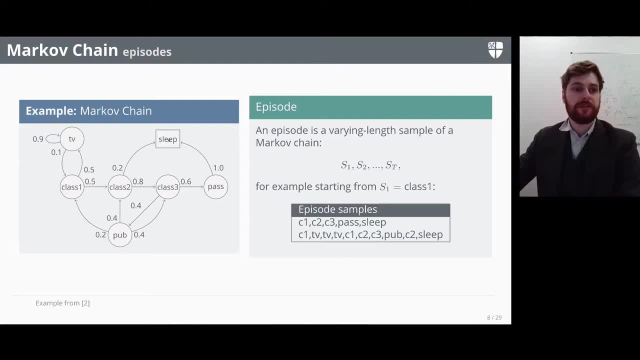 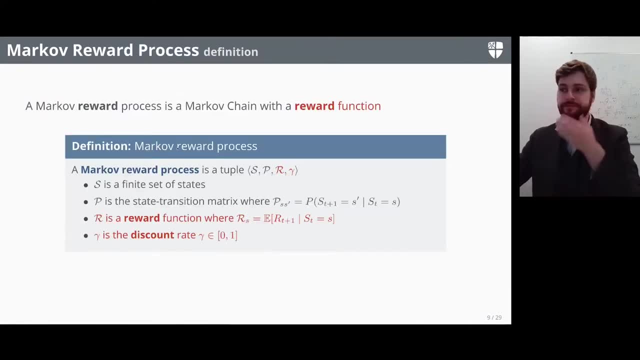 a, you will always reach this terminating condition. So that's a Markov chain, and the Markov reward process basically introduced the notation of rewards into this Markov chain. So it's a Markov chain, but we additionally have what's called a reward function and the rewards are: 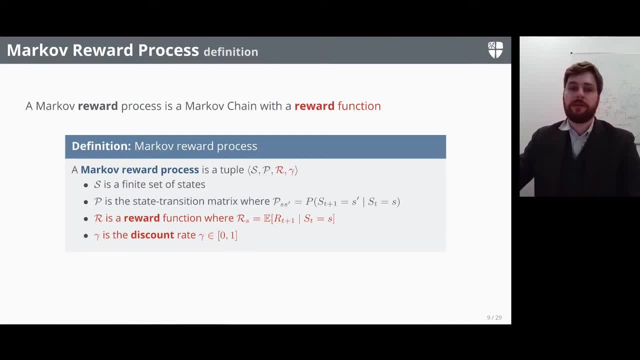 it's just some function which gets a reward. For example, it could be like extracting some pixels from like a games display. it could be like extracting gold from the game states. but if we recap from like what we touched on last week, we said that at each time step t. 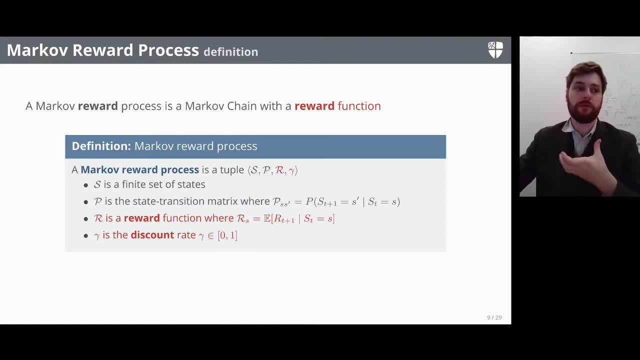 there was just this scalar signal which was called the reward. So we had those examples where we talked about time-based goals, where you might like lose reward every time. step we might have like the forward motion of a robot, or in chess we might have just. 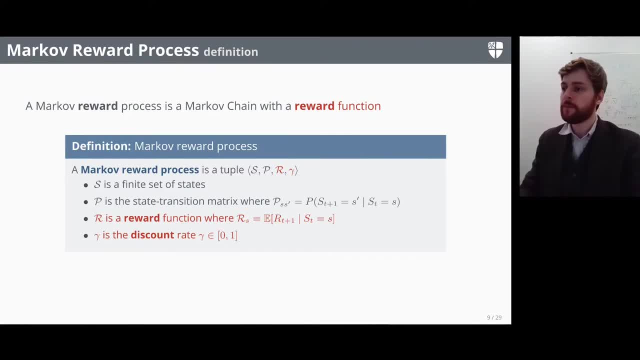 reward only when we win and we get checkmate, um, or you might have like multiple goals and if you've got multiple goals you need to sort of balance your awards out carefully for your decisions. and then do you remember we talked about briefly how designing rewards was actually a challenge. 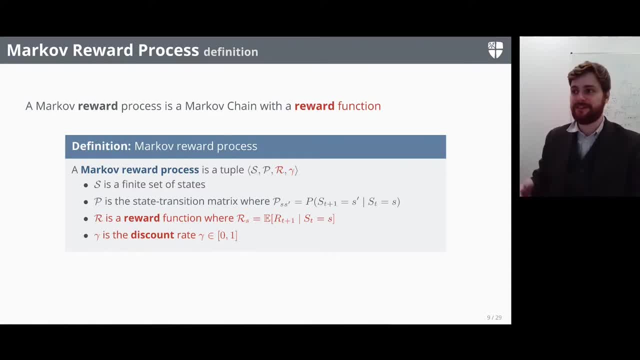 and we talked about, like demeter's touch in greek mythology, where you know he has this idea but it doesn't turn out well. so formally, uh the r is a reward function, um, where the reward at a given state is the expected value of, uh, the reward conditional on the state. okay, and there's also 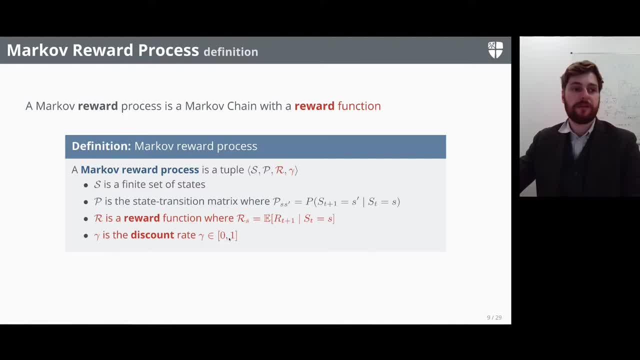 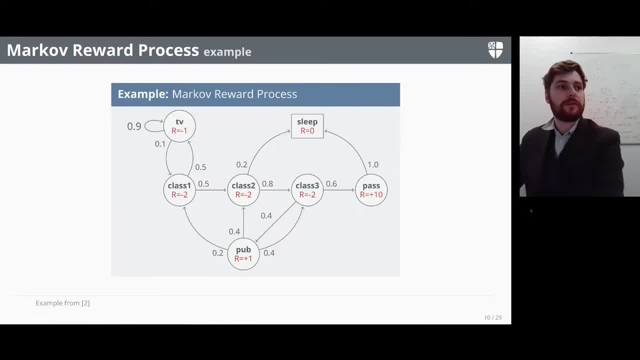 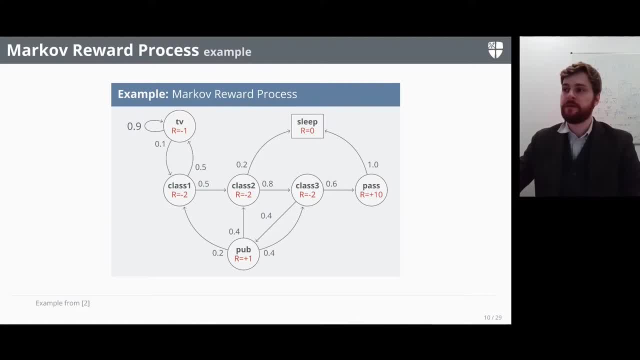 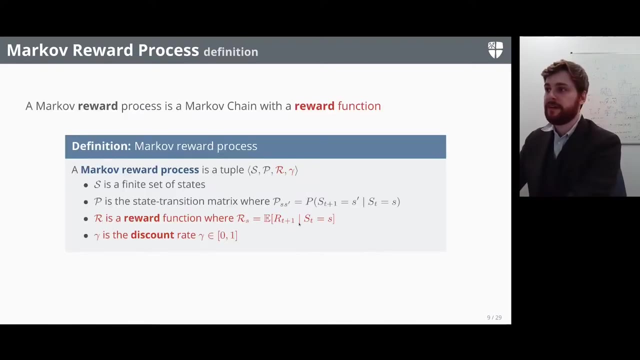 and here the red values are to be basically read: upon entering the state, i'll receive, receive a reward of minus two from the environment at rt plus one. this, this idea of, if we go back to the definition, this sort of rt plus one- here is actually saturn and barto notation and it's kind of done on. 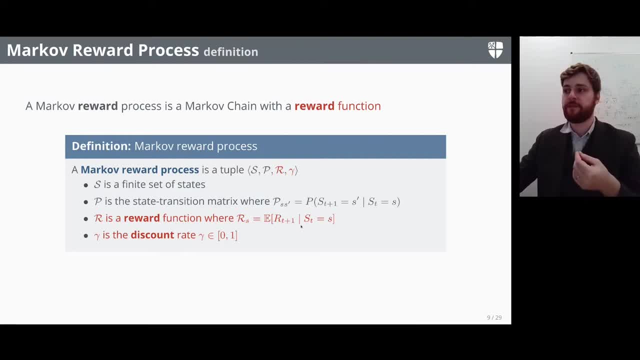 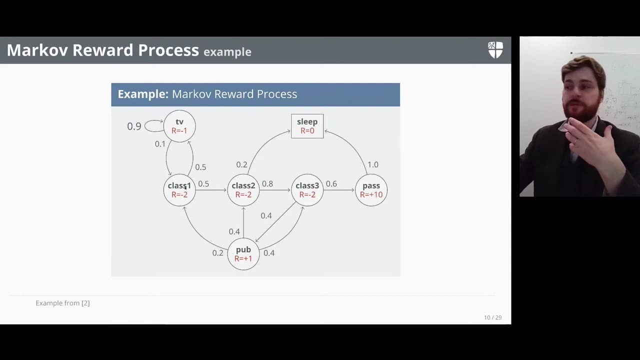 on purpose to denote the boundary of changeover where the agent receives the reward from the environment. and then, if you remember we talked about, it was the environment that gives the reward, not necessarily the agent. so we would say, upon entering class one, the environment gives us the reward negative two. upon entering class two, we get given the another reward of negative two. 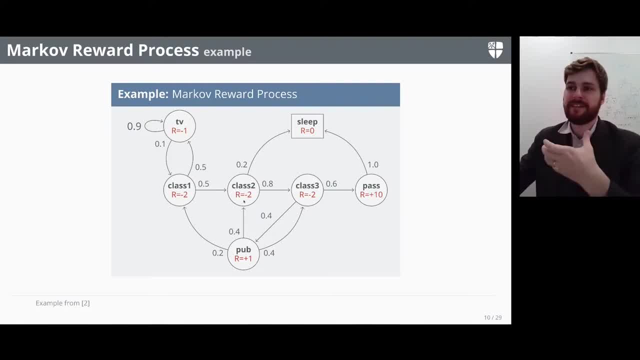 back from the environment. but basically it's kind of like the immediate reward. so a lot of people are confused by this idea that rt plus one is considered the immediate reward and some literature actually does go as far to define it otherwise. but again it's just Sutton and Bartow notation and it does make sense. it really helps drill in the idea that in these 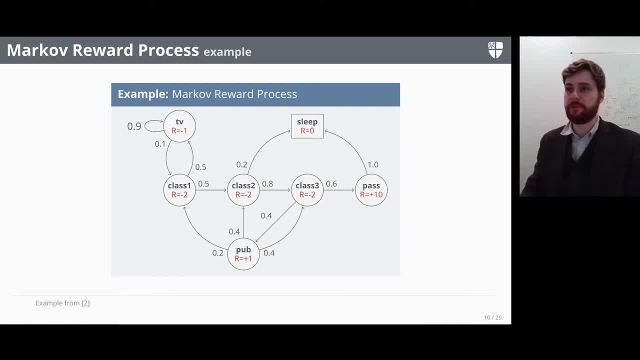 formalisms. we're talking about the environment, giving us the reward back to the agent. okay, so in this case here we don't really want to have this cycle where we keep getting positive reward here so we lose reward by watching tv, even though it might be sort of enjoyable in. 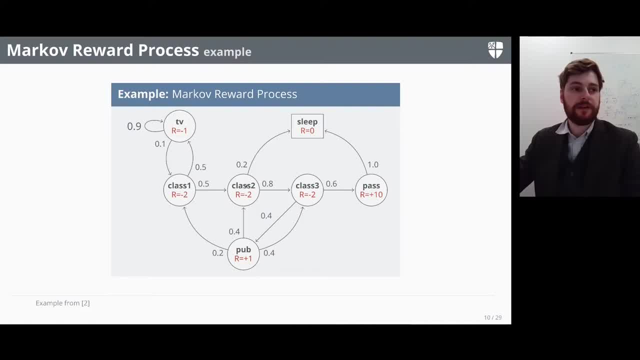 the short term, but every time we go to the class it's pretty tedious usually, so we lose some reward. going to the pub's quite good though, but then you've still got to go back to class at the end of the day, and then, once you've passed, then you get a big burst of reward and you can sleep. 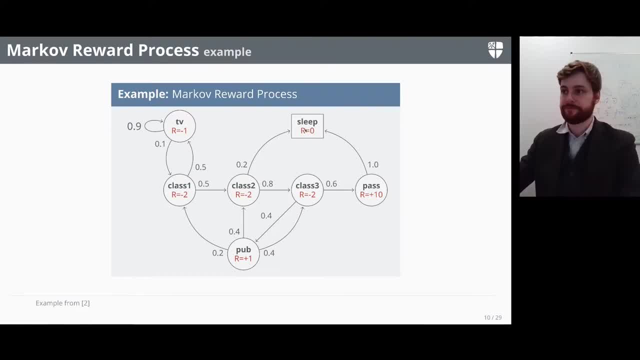 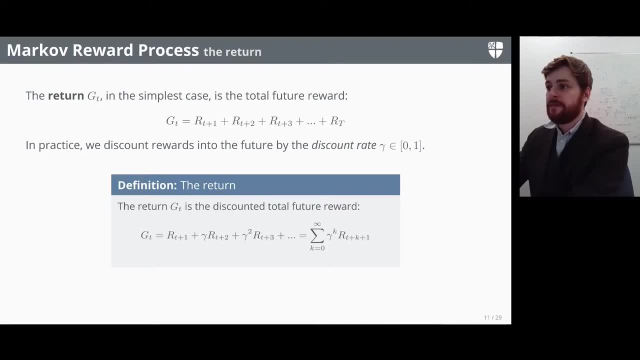 once you've terminated. that's it, that's the end. so the return is well, the return, really the future reward is called the return, the future reward, and it's parameterized by this discounting factor or this diminishing factor, gamma, and gamma is typically a scalar less than one, where we have gamma to the power of. 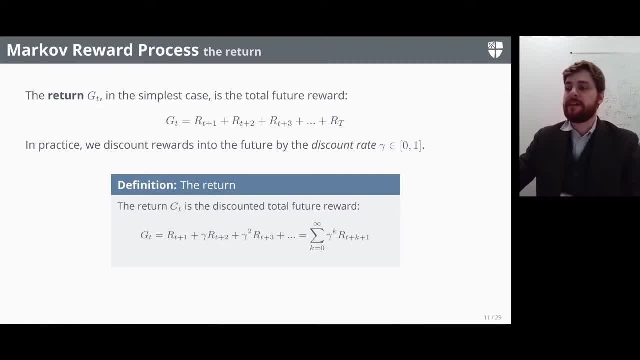 k for the k future time step. basically, we may wish to penalize rewards far into the future, so so the return is just sort of all of the rewards going into the future. so if you play an episode of a mark of reward process at every state, we're going to basically want to sum up. 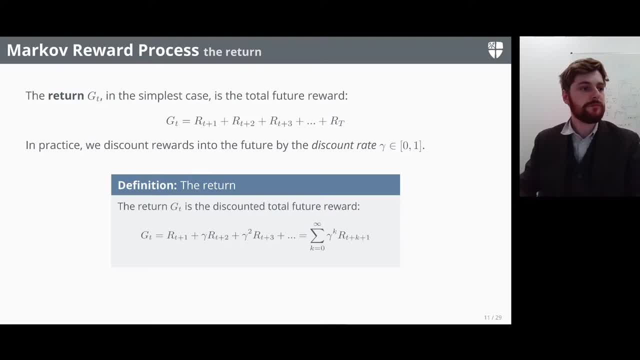 all of the rewards going into the future, and but when we're talking about the return, there's lots of reasons why you you might not want to just like have all of the future rewards counted equally. that would be quite sort of long-sighted behavior. so we might want to 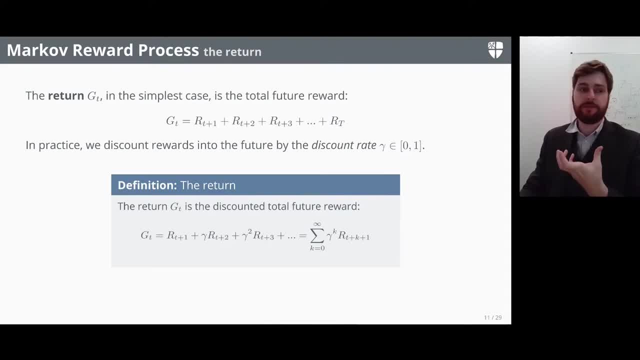 penalize it for various reasons. so if we were to set gamma to zero, then you can see this: this is just going to zero out this term, which is going to zero out this term, and so we're only going to be counting the immediate reward if gamma is zero. so we're going to have this kind of short-sighted. 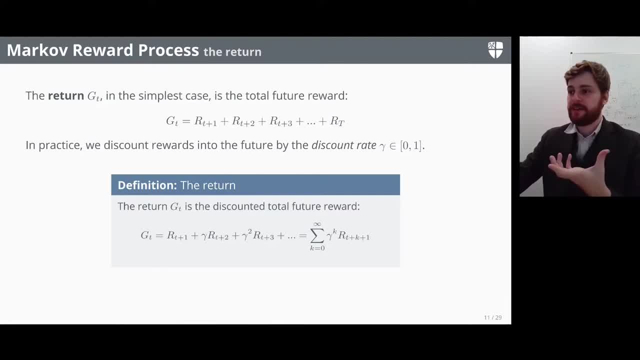 not very intellectual agent behavior. whereas if we were to set gamma to one, then gamma to the power of k or one to the power of k is equal to one. so all of the future rewards are going to be counted with equal weights. so that's this kind of far-sighted evaluation, so you can kind of 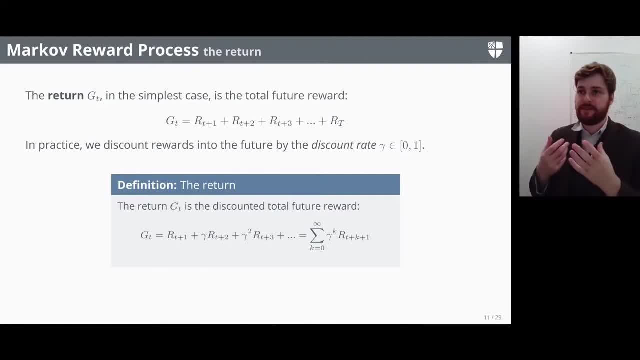 think of it like if you just like set gamma to zero, it's a bit like being a kind of a heroin addict. you're going to just get your immediate burst of reward and then detrimental to all of the negative consequences that will have into the future of your life, as you get. 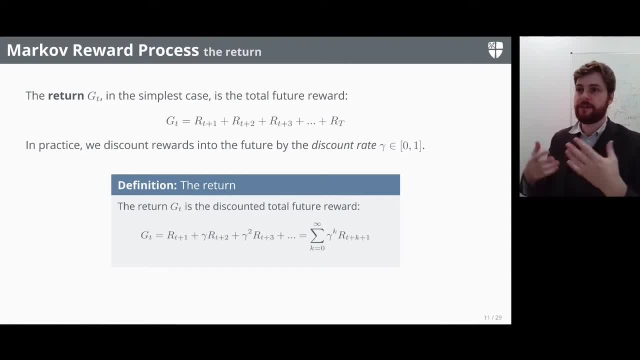 addicted to heroin and just keep injecting yourself and everything fails, your career fails, and so on, whereas if you've got that like long-sighted reward, where you set gamma to one, all of the future rewards have equal probability, which means, if you have a very long episode- so maybe this, this, is representing your entire life- then, um, it means you're going to 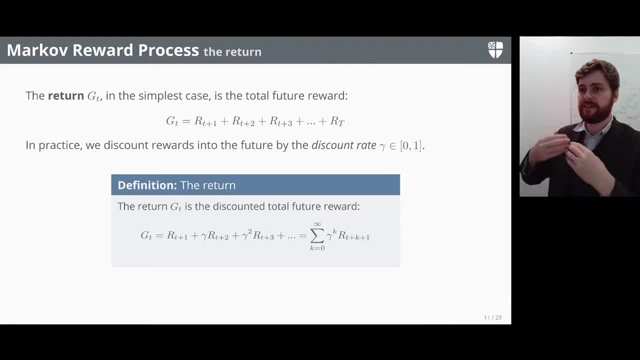 sacrifice yourself crazily in the now to maximize your long-term rewards. so maybe you'll just like study, study, study, study, study. never meet anyone, but you're going to be, have a very successful career or so on. so you can kind of think of it like making your agent have various political or religious 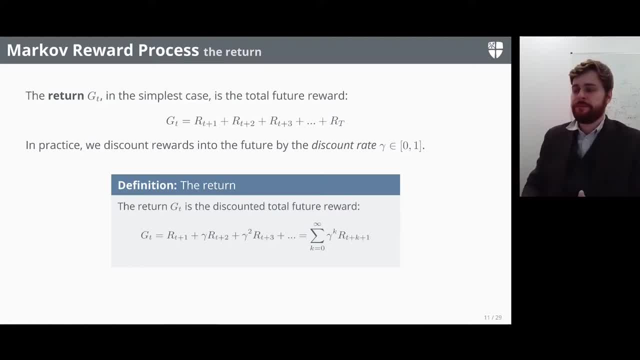 incentives. um, however, the uncertainty does increase in the future. so, um, so we can't really model the future. so we can't really model the future. so there are actually quite good reasons to not have gamma so high as one, but to lower it a little bit, and actually mathematically it's 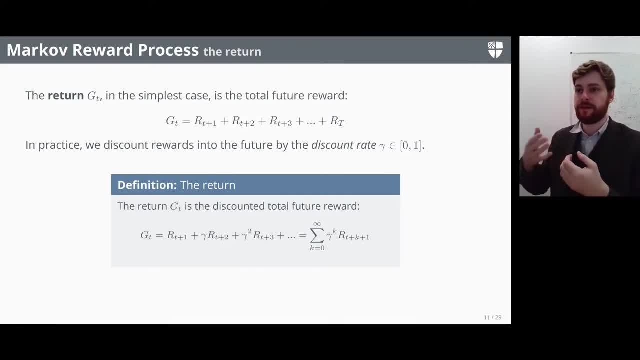 convenient, so you will get better performance because you'll have shorter episodes if you're, if you don't need to go so far ahead. another nice thing about this discounting factor is it helps us handle infinite loops in the state transition graphs. so if there are like infinite, 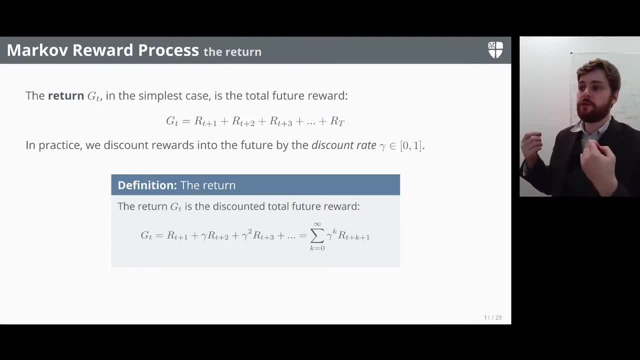 many states in the markov chain, then the return will always be finite if gamma is less than one. and also there's like a biological motivation behind this discounting factor, which is that if you actually look at animal and human psychology, we actually have preferences ourselves to. 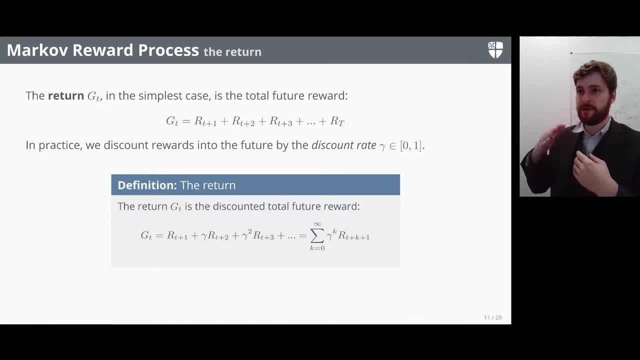 immediate rewards. we tend to have our own slightly lower gamma internally, which helps us to chase after short-term goals. we're not very good at chasing after very long-term girls and having master plans, like elon musk does. so, um, that brings us on to the state value function. 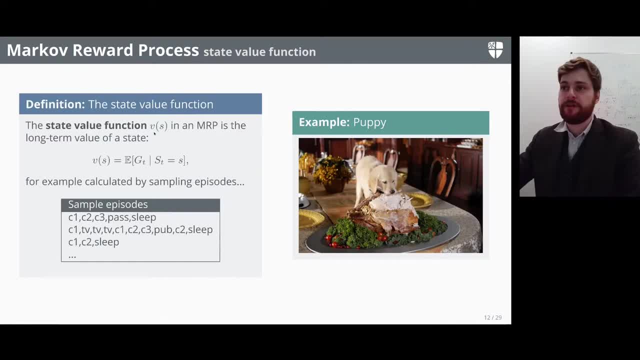 or the value function, and this is a really central idea in reinforcement learning. so the value function in a markov reward process is the long-term value of a state. so every state, you can say, has this value function which is defined as the expected value of the return, conditional on some state. so every state. 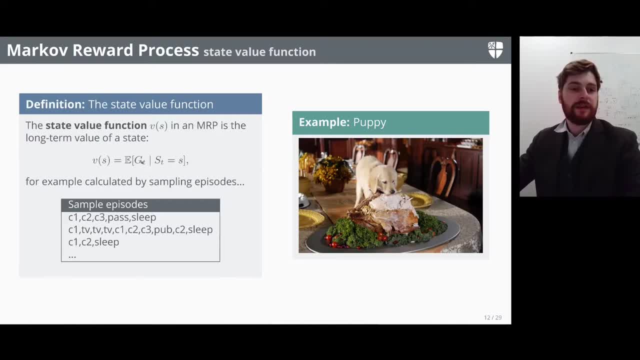 has this expected value of the returns and this is really calculated by sampling lots of episodes and averaging. so if we consider this puppy here, it's really enjoying the reward now and it's in quite a good state here, but maybe this state to be in it's not like as good a state to be in as the puppy. 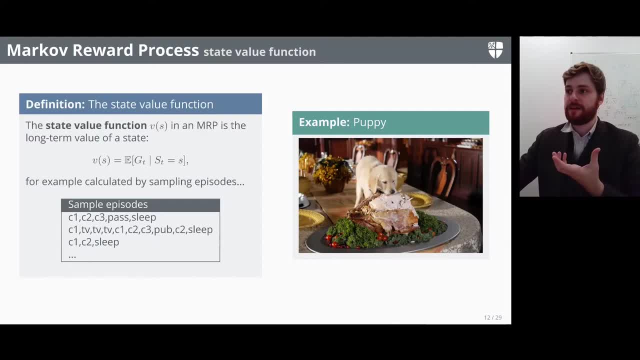 might think, because in the future this state might involve the owners having to discipline it. it might not get dinner, even though it's just had a similar like taste of the thanksgiving meal or whatever it is. so the expected long-term value of this state for the puppy isn't actually. 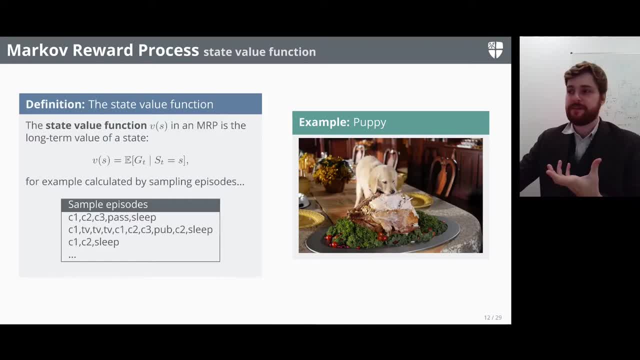 that particularly low because on average the owners are going to discipline this puppy where i'm going to be angry at it. so the the value function is really a way of saying what is the value of being in this state on expectation, from where i might end up by going from this state. 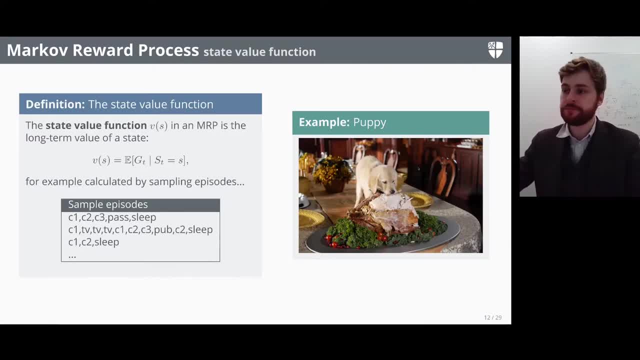 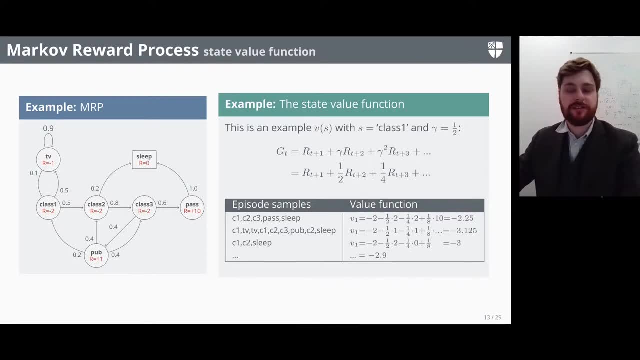 what is the long-term value of me being here? okay, so let's try to look at some examples. so this is where we try to look at the uh, the value function, uh for s, and we're just going to sort of say what is the value of being in the state of class one? so if we say, uh, gamma is equal. 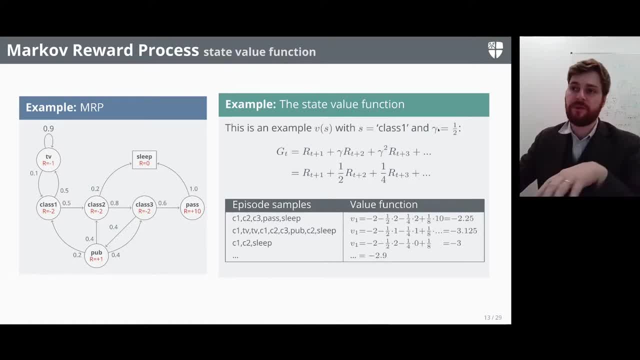 to a half, so it's kind of not necessarily immediate reward, not necessarily fully long, far-sighted reward. then if we take our definition of gamma- sorry, of the return, the discounted return, gt, and we plug in half, basically now what we do is we we have to sample lots of episodes. 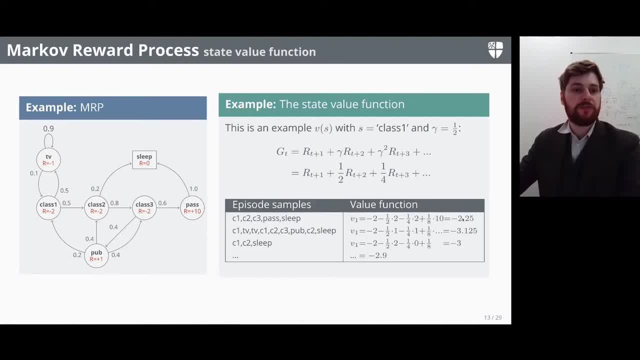 and we can then begin to compute the value of the return here. so, for example, if we've got here's one episode where we go class one, class two, class three, pass and sleep, then we take the uh reward of minus two for being in class one. that's over here. 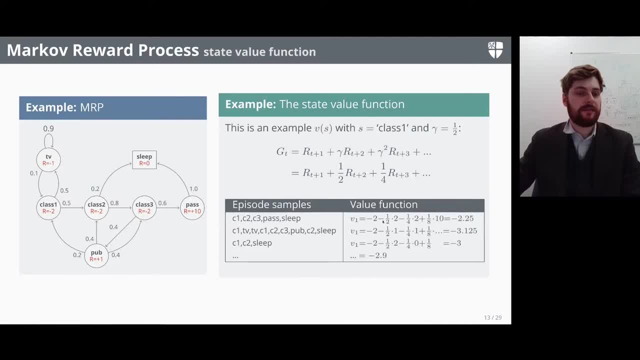 and then we add: uh the well, in this case we're negating because we have a negative reward, the reward of class two, as it's discounted by gamma. and then we keep doing that. so then we add on the reward of being in class three, discounted by gamma, which is now a quarter, and then we add on 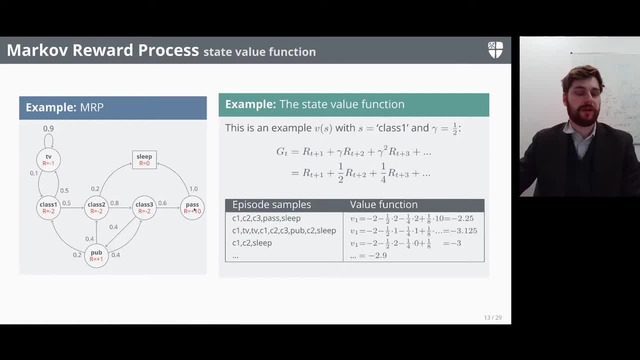 an eighth of- because we're now gamma to the power of- i don't know what it is- but um, an eighth now, uh, of the reward of being in class 10, and then we're in our final episode, which is just zero. um, so if we add up all of those values, if you plug this in, you'll get some value of negative 2.25 for. 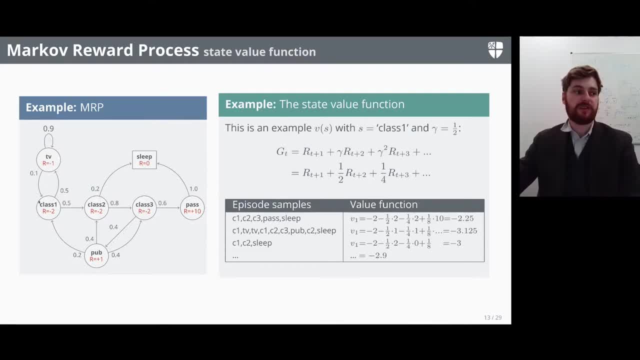 being in this state for this episode, and as you just randomly sample episodes from class one, you're going to get different returns as you go through them. you sample through the episode. so here's another episode from class one, here's another episode from class one. so you get like lots and lots of these returns out of it, and then the value function is: 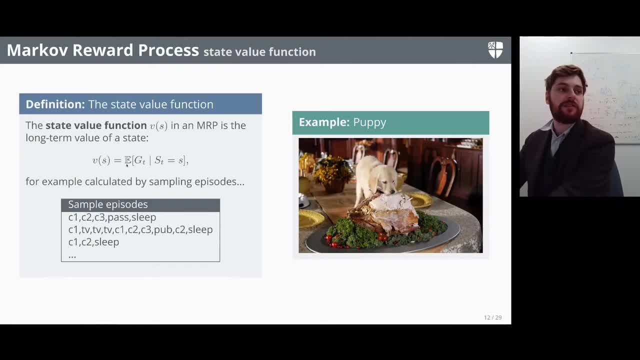 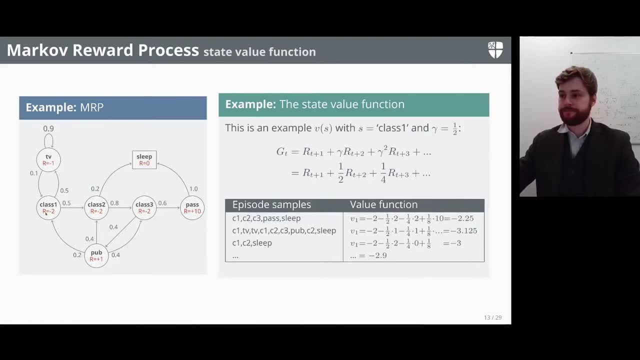 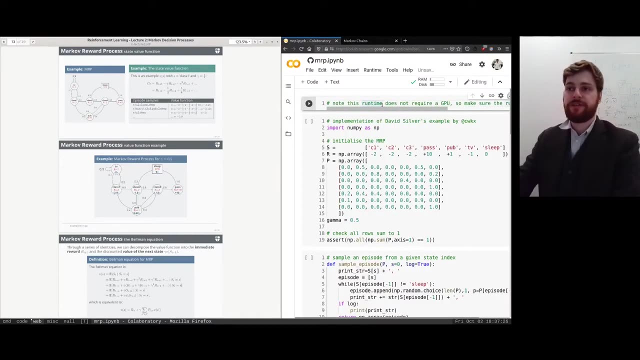 just the- if you remember the definition, it's the expectation um of those. so it's just really averaging all of these returns and you will end up with some value for this. so i think i've got a demo of this so you can access these. get demos from duo. you can just click like the collab link. 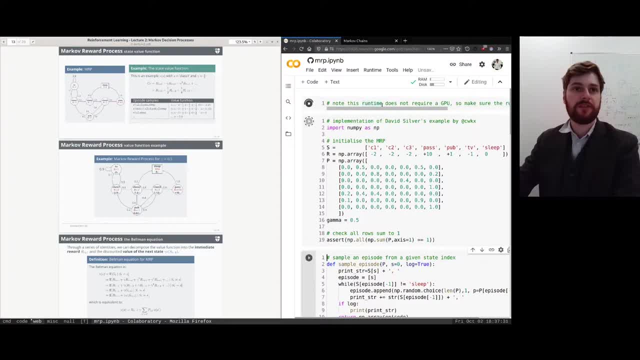 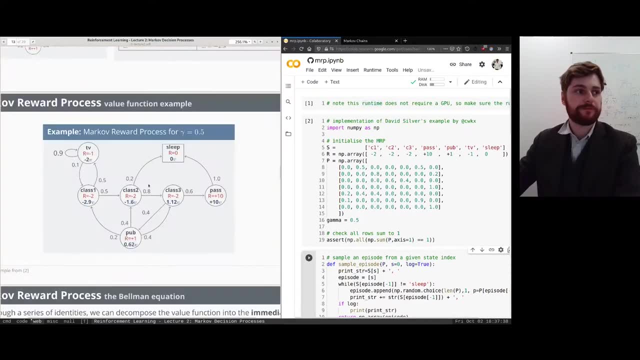 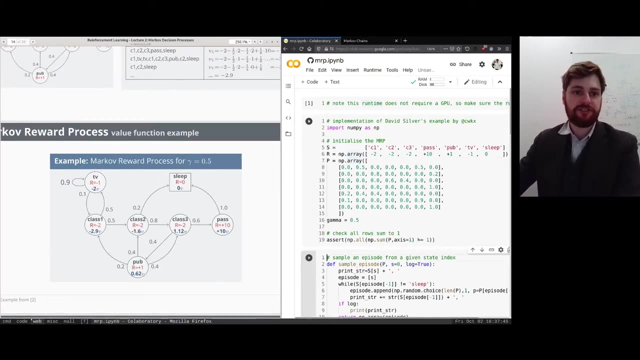 next to the corresponding lecture materials. so i'm just going to here define our states, which is just straight from this example and, um, okay, so let's just run that, and this is just checking that. they will sum to one and then we're going to have this function here, which 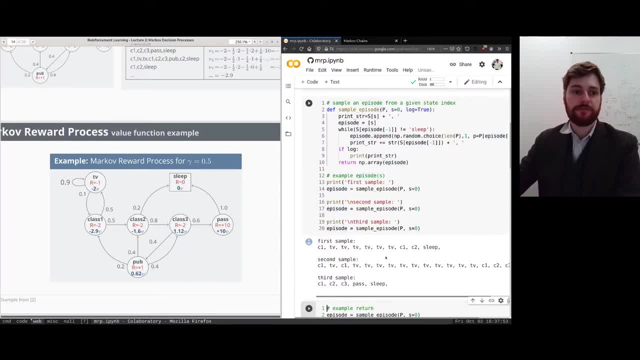 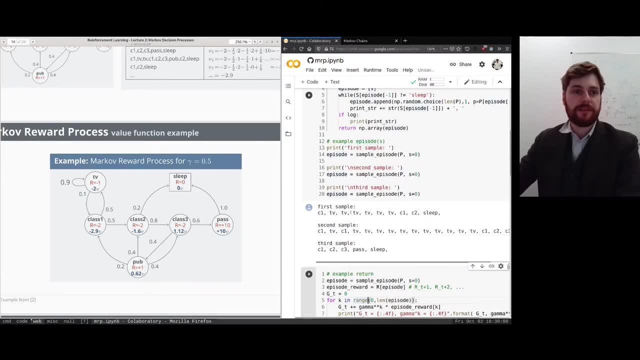 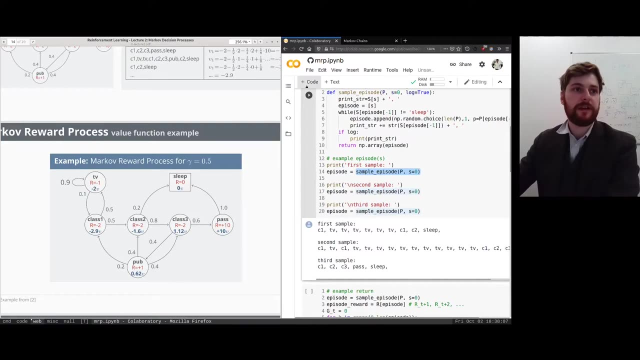 a samples some episodes. there we are, we have some nice samples, and then here we're going to, um, just basically, so this is just sampling this markov process here, just as we've seen, and we can actually just uh, type, sample episode as many times as we like, let's just do another, just so. 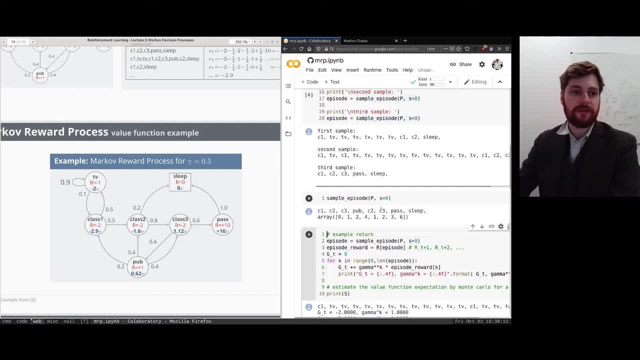 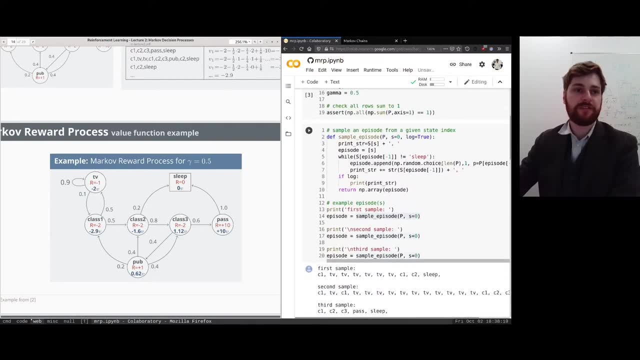 you can see it. so here's a. here's a sample of an episode and you can just run this as many times you like. under the hood it's using like numpyrandom choice, so it's just working out when it should transition based on the probabilities as defined by this straight. 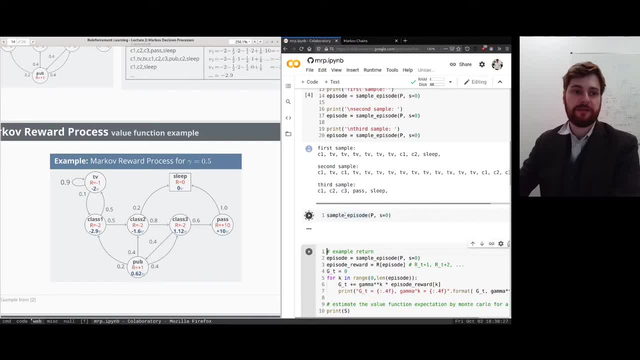 transition matrix and you can just sample this as many times as you like. yeah, that we've got a really long one now which just watches lots of tv. that's a huge amount of tv this guy watches. oh, there's another long one, see if we can get a short one. and there's a short one that looks like. 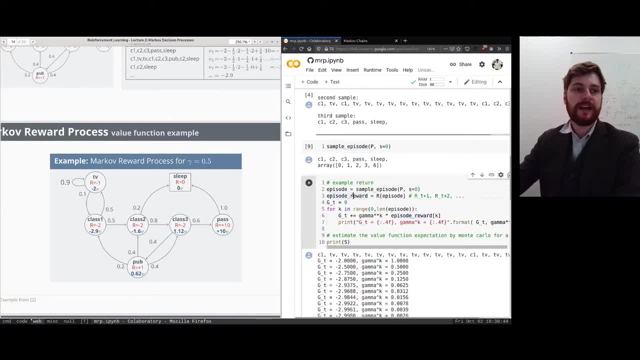 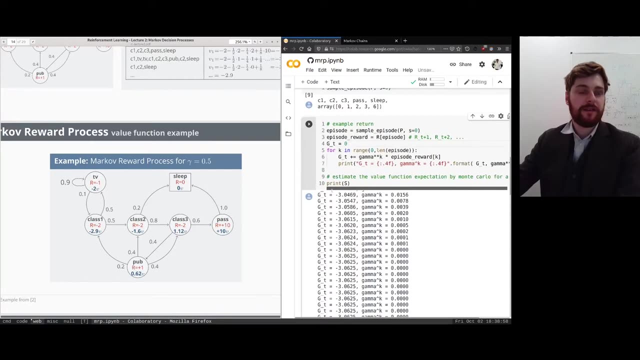 an optimal one, actually. so now, how do we compute the value of being in class one? well, really, um, we just uh, need to keep averaging it. so it's actually a monte carlo method. um, so let's just run through what's happening here. we're sampling an episode and we're computing the reward at that episode. 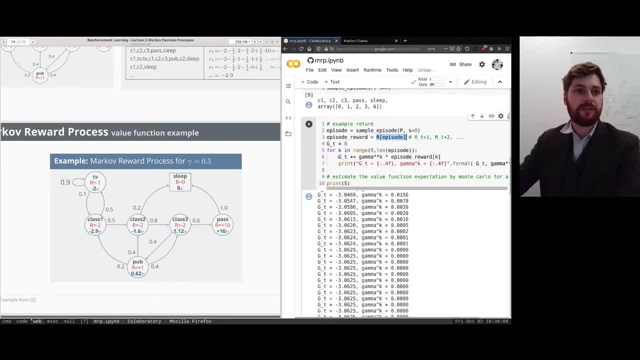 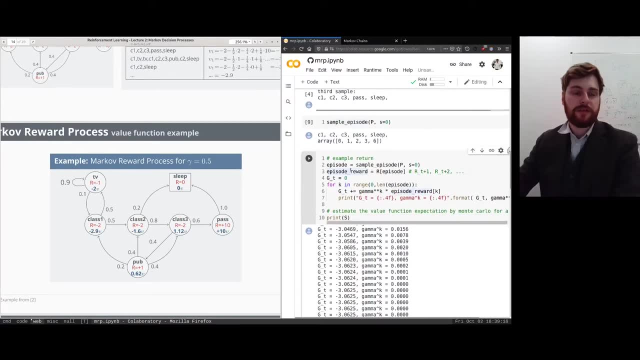 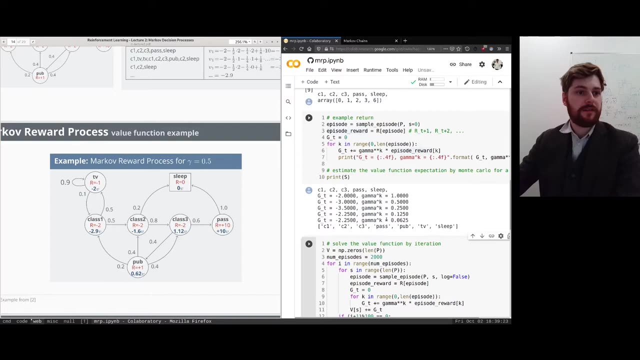 and then we're going to just go through the entire episode and compute the return as per the equation. okay, and this is quite a long episode. let's see if we can find a short one. so this tells us the return for this episode here. okay, so how do we solve the value function? well, we're just going to solve it. 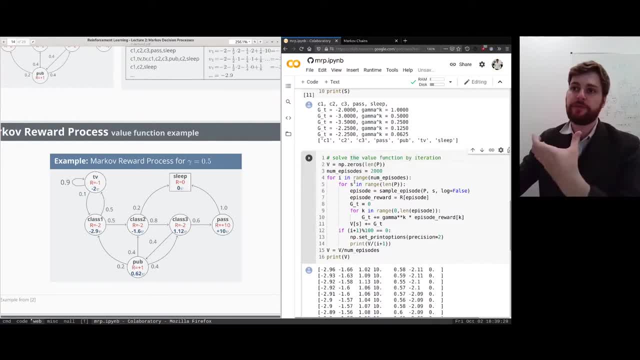 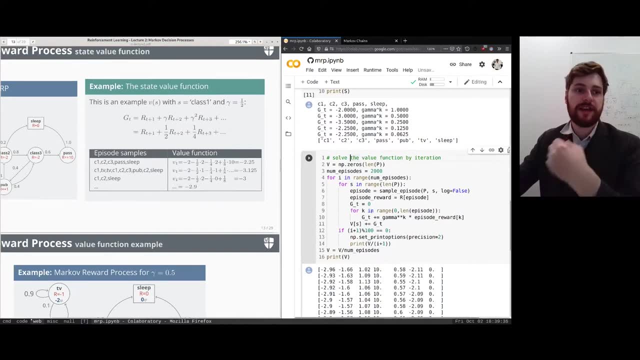 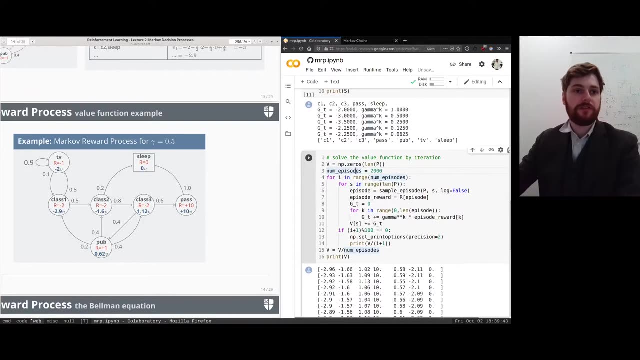 iteratively. so we're just going to do lots and lots of samples. and then we're going like in the table here we're just going to do maybe hundreds of samples or thousands of samples and we're just going to average it all together. so here we have- um, we're going to go through lots and lots of. 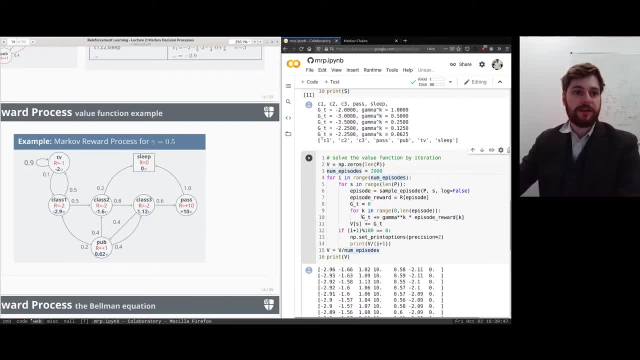 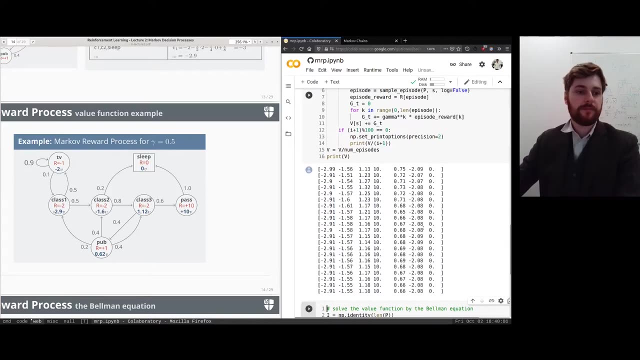 episodes and then, for each episode, we're going to calculate the return, the discounted return, just going to divide or average by the number of episodes. so let's do that, here we go. these are all different episodes and this is actually for all of the states as well. so this is the value, i believe, for 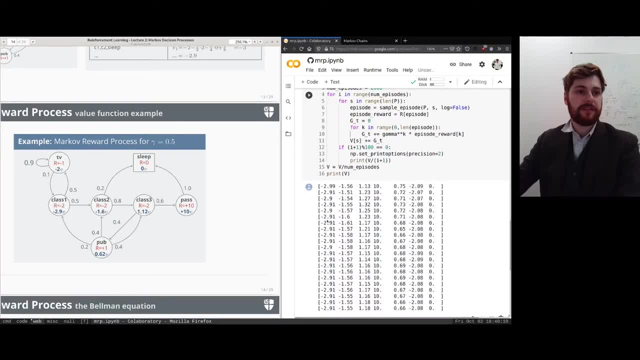 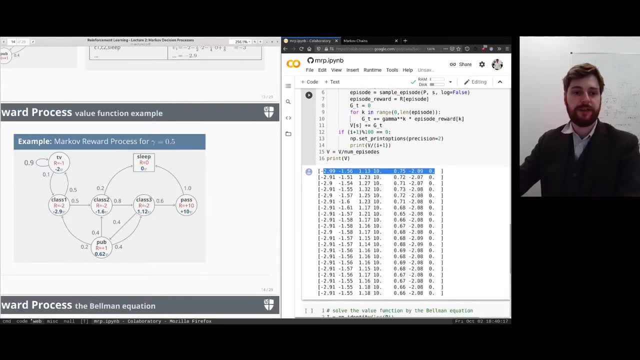 one of the first states. okay, so this tells us the value for all of the different states just by this iterative averaging process and you can see how at the beginning it sort of starts off not very good and it starts to converge on the true value, function over lots and 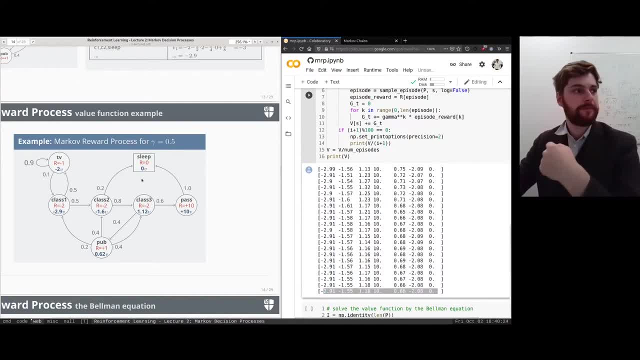 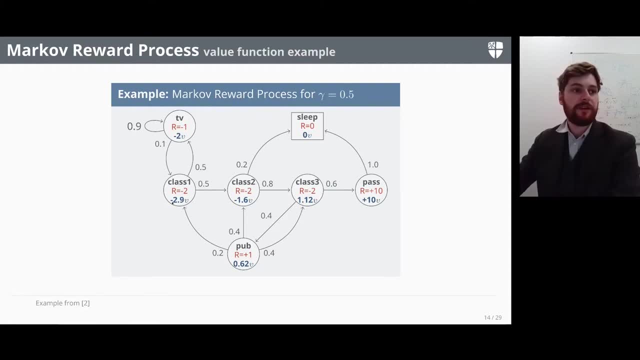 lots and lots of trials of different episodes and lots of averaging. okay, so if we put that all together we can say that if we can actually compute the value of being in every state so we can see just by eyeballing these values, the best state to be in is this past state, where 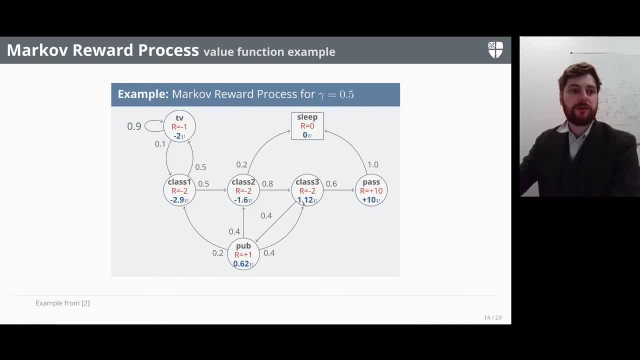 we've got both value, then it's quite good to be in class two. we've got like 1.12 then, then it's not quite so good to be in the pub And it's really not that great to be in class two. negative. 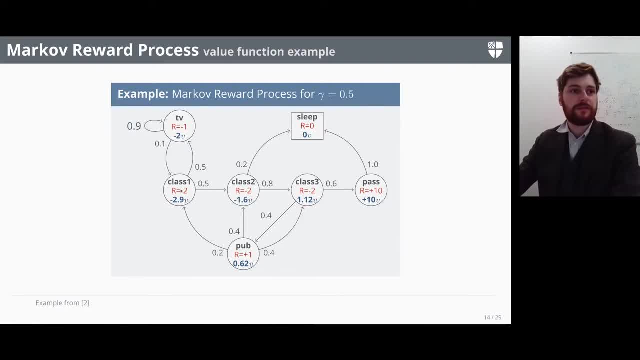 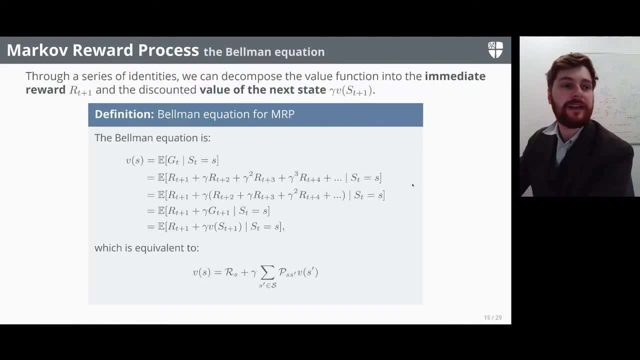 And it's really bad to be in class one and so on, And then at sleeping we have zero value. OK, and now this brings us on to another really central idea of reinforcement learning, which is really where a lot of the advances in this field have come from. 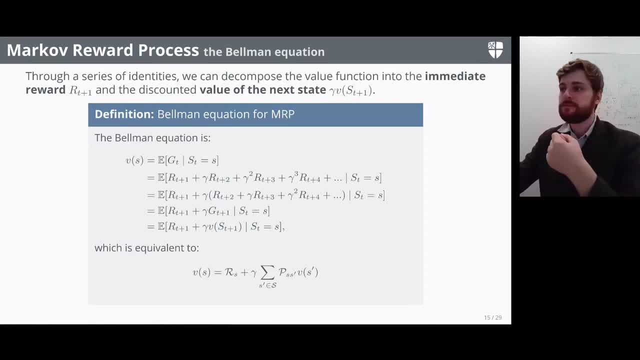 which is the Bellman equations. So we want to know how good it is to be in a particular state, We want to know the value of the states, as we saw, And the Bellman equation really just follows a series of identities. that rearranges that value function definition. 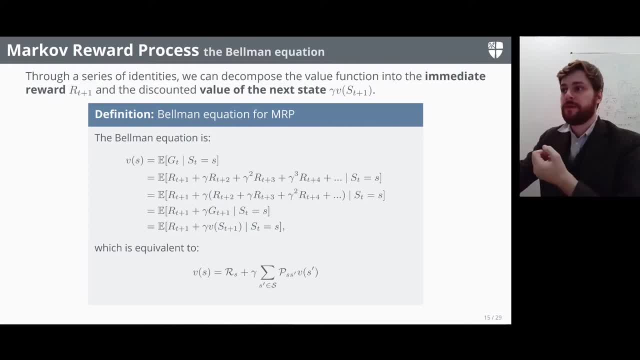 into a more localized and efficient form. So if we just kind of read the equation as we go down, we say that the value function is the expected return, given the start, given that we start in some particular state. OK, that's just the definition of the value function. 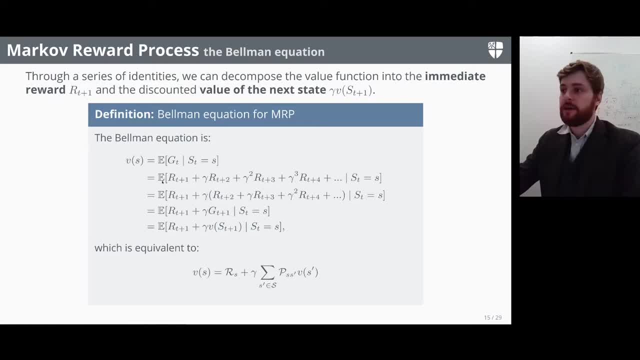 as we've already seen it. So we could unroll the definition of the return. So we already defined what the discounted return was, So we can just plug that in So we could say it's the sum of the rewards going into the future discounted by that gamma rate, gamma. 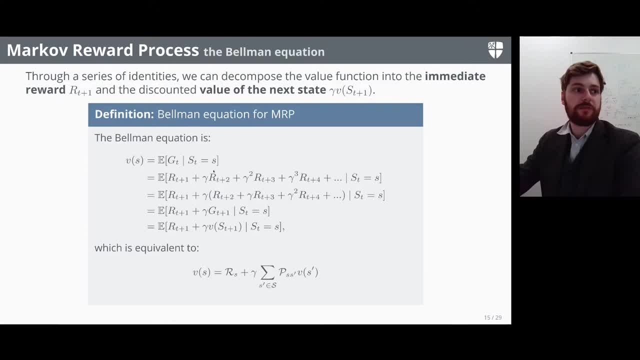 OK, and conditional mean the state. So we've already seen that. We've substituted that in. Then we can actually factorize this just by looking at it. So we could actually pull gamma out OK, And we could pull it outside and factorize it there. 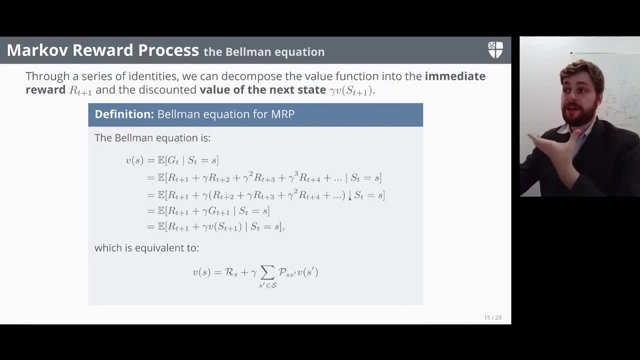 And now you can see we have the definition of the return again. So you can see that from this we've actually got inside here another sort of mini definition of the return, But instead now we're starting at the next time step of gt. 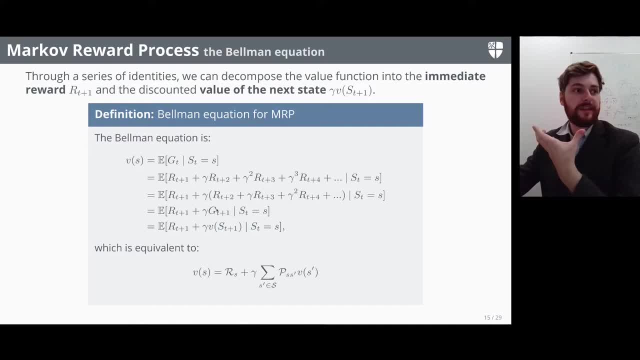 plus 1.. So all of this part here is just the same thing as saying it's the return at the next time, step OK, And that actually brings us on to the final part of the Bellman equation. But it's really just saying it's the immediate reward. 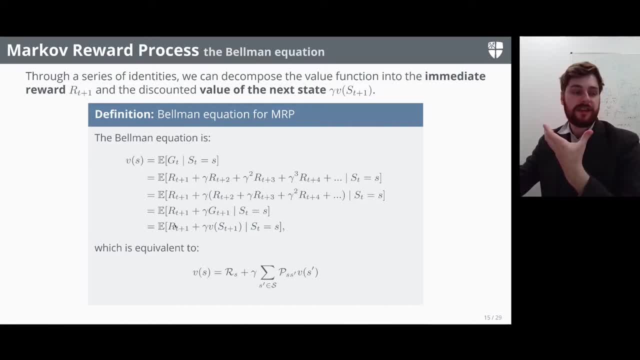 plus the discounted return at the next state, which is the same as saying it's the immediate reward plus the value function at the next state. I don't know if you remember the- maybe I can put this down from our previous lecture- the definition of the expectation. 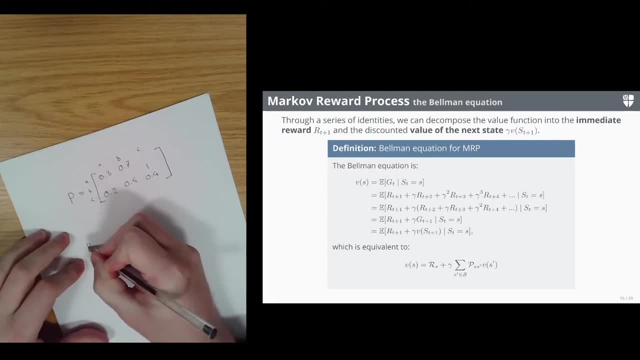 We said that the expectation of some random variable x is equal to something equals 1, all along little x times the probability of gt. OK, So that's it, Thank you Bye. Little xi times the probability, So we can actually integrate with respect. 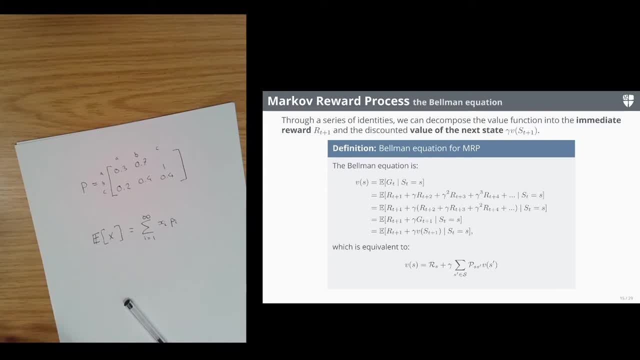 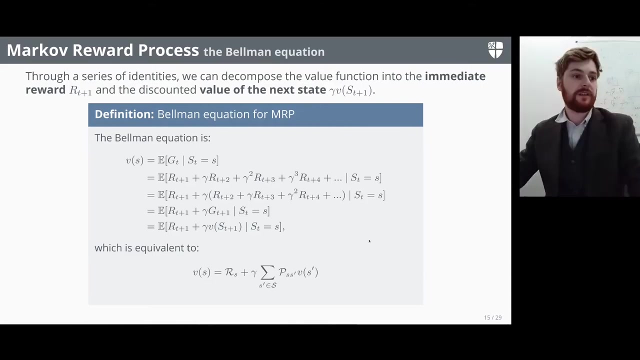 to this probability, the next state. so the value of the transition, replacing that expectation here by summing all of the discrete kind of states, the probability times the value function at the next state. So so that leads us into this equivalence here where we can just say that the value function is. 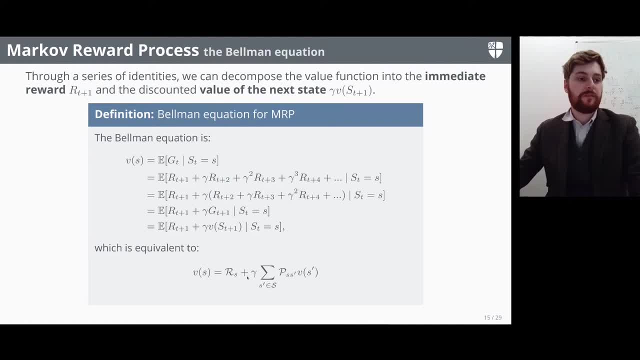 actually equal to the reward at this state, plus this discounted idea where we sum all of the next states transitional probabilities, so it's summing all of the probabilities transitioning to the next state. so we've kind of broken down that idea of the return into this sort of immediate look ahead. 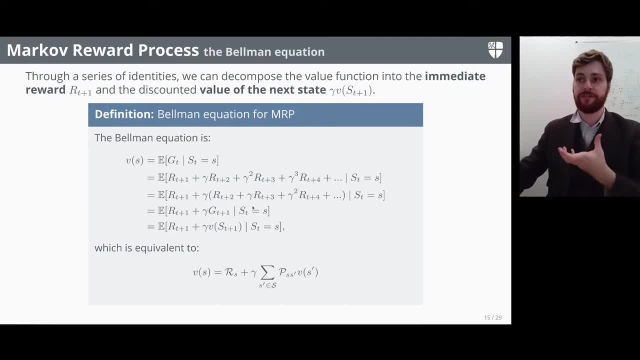 idea of the value function. so we still need the value function at the next state, but we've decomposed it so we've now only got. we can compute it locally. so just to read what we wrote here: for a series of identities we can decompose the value function into the immediate reward. 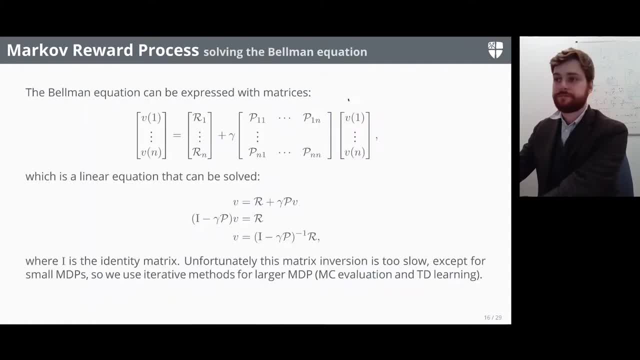 and the discounted value of the next state, and actually this can actually all be expressed with matrices, which is actually a linear equation that can be solved. so it actually requires a matrix inversion and let's just go back to here. so, yes, you need to invert the matrix. 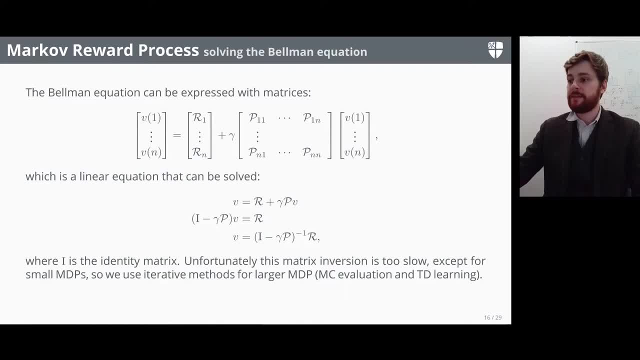 but you can kind of read about that. and the matrix inversion complexity is about o n cubed. so you can kind of read about that and the matrix inversion complexity is about. but there are quite more efficient ways to do that matrix inversion. you can read on wikipedia about the kind of asymptotic complexity of the bounds. you can. 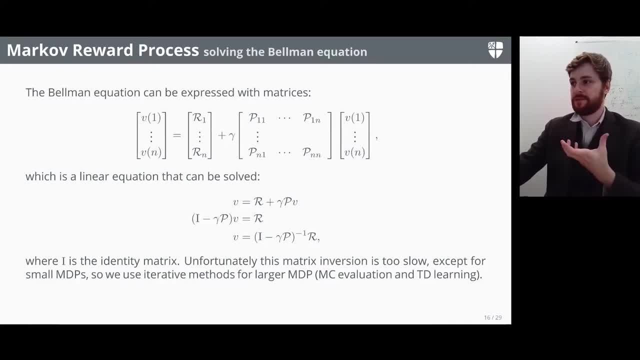 actually reduce it to o, n, to the 2.3 something around there by the coppersmith winograd algorithm. however, in practice these have really high constant factors, those kind of like matrix inversion libraries. so it really is on cubed out there which and you would use like blast and alpac and they do like numpy cores and they're. 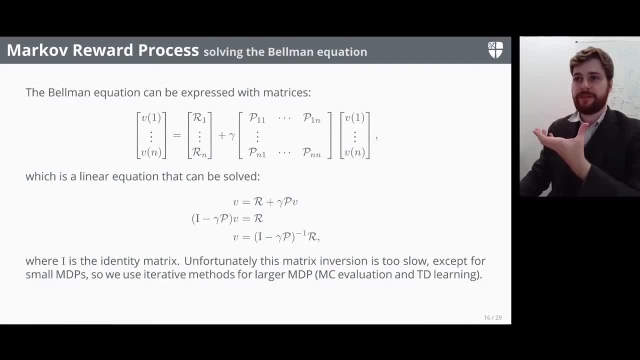 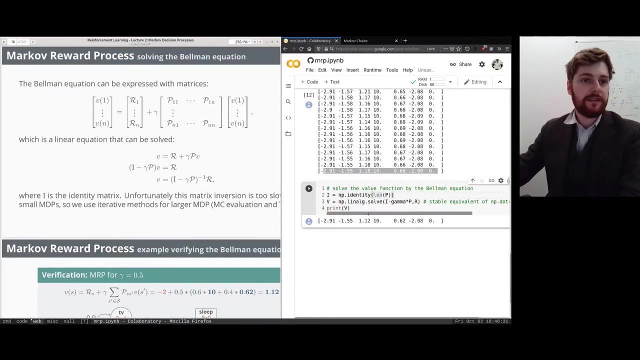 hand tuned to really outperform the theoretical coppersmith winograd algorithm. so you really have that bound in there. so unfortunately it is quite slow, except for very, very small mdps. but i'll just show you in the code here what it means to solve that linearly. so this, just this, basically shows it. 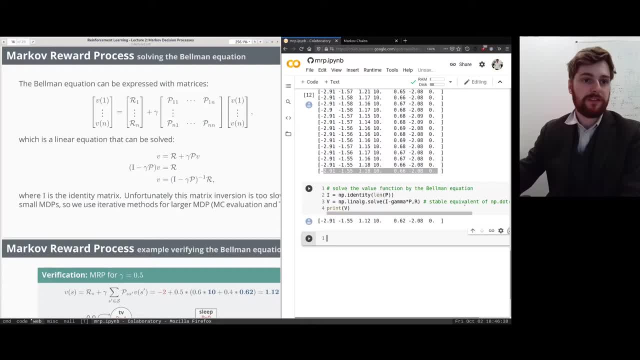 if we plug this in directly into the matrix inversion and then we can see that it's actually directly. we can solve it using the library which is. i've shown the equivalence there. but this is just the solution output which tells us the value function for all of the states. but that's just not. 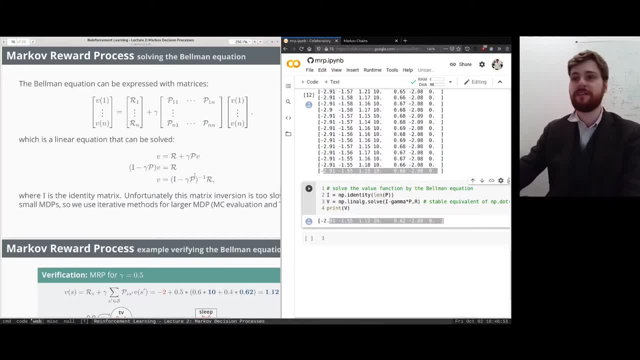 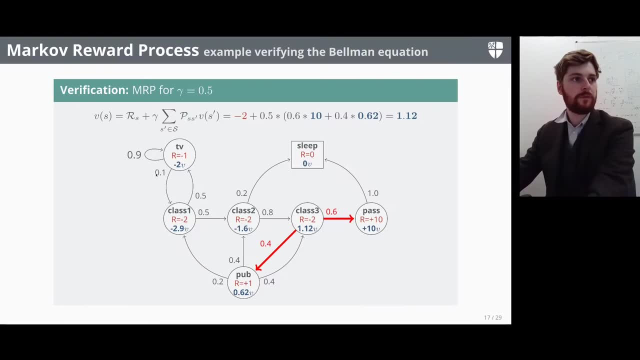 something you can do with a very, very large state transition matrix, but it's nice to just see that it can be done. there's a nice close form solution for it. so should we actually verify this? let's verify this value function here. so it's quite cool because we can actually estimate the value of a state. 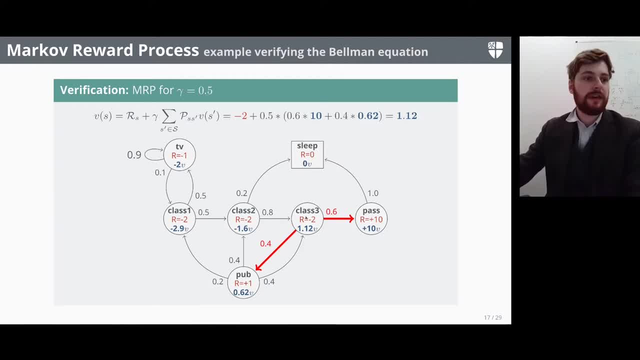 far into the future, just by its local conditions. so here, if we look at class 3, the value function 1.12 according to the bellman equation. we can see just by the definition it's the reward plus the discounted value of summing the state transitions to the next state. 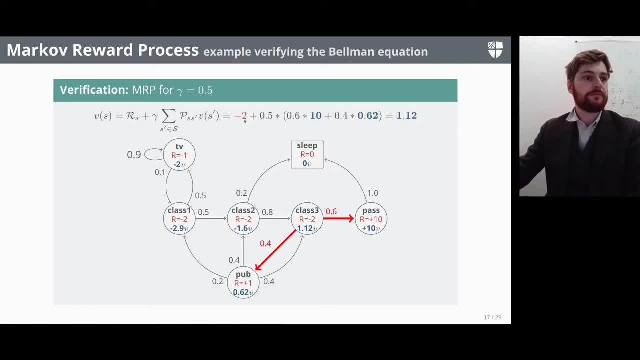 so that's just equal to- let's start here- the immediate reward, which is minus 2 of this state here plus the discounting factor gamma, and we're just setting that as equal to 0.5. so that's here times, and then we're going to start by saying it's 0.6 because we're summing over the transitions. 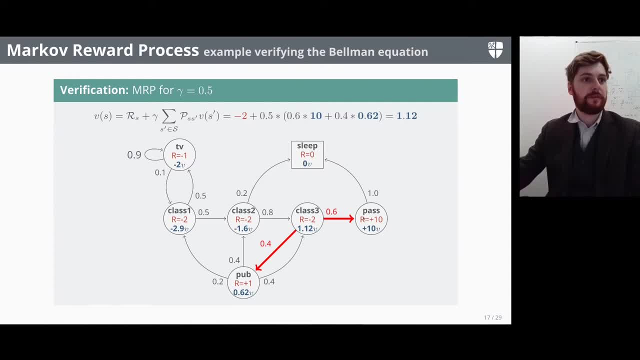 the probabilities. so it's the probability of transitioning to the, to the past state. so it's 0.6 probability times uh, times the value function at the next state, which is this 10v here, and then we're also going to sum, so we're going to add also the probability of transitioning to. 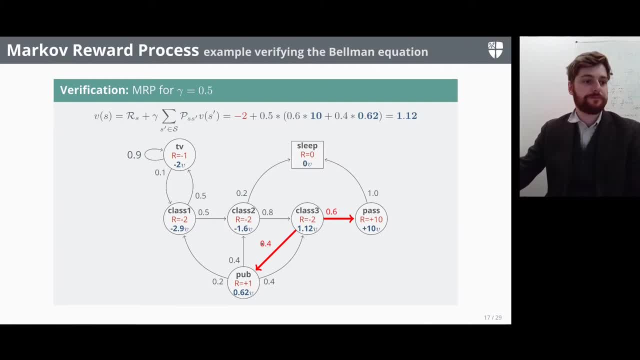 this state, which is 0.4, and that's the probability times the value of this state, which is 0.062, and if we evaluate all of that, we get the actual value function, which is 1.12, which we can, uh, confirm is true. okay, sorry. so that helps us to verify very quickly that this is. 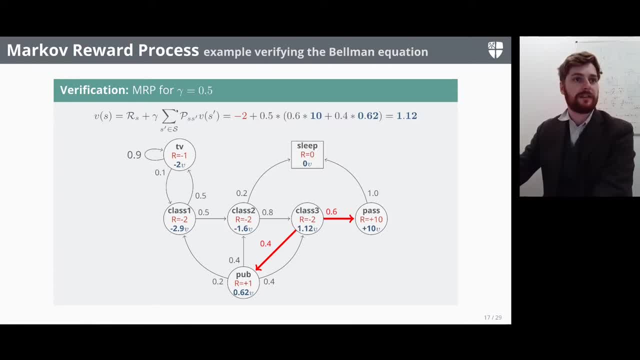 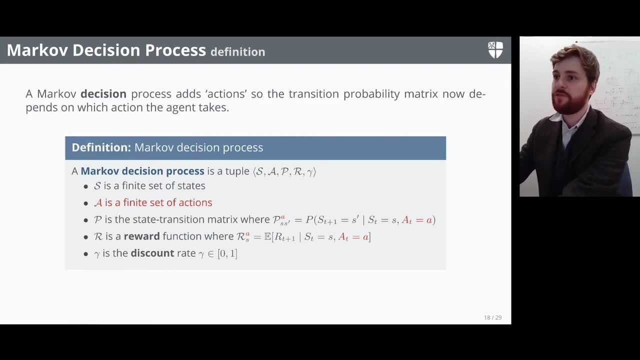 truly the value function just by the bellman expectation equation here. okay, so now we can actually move finally on to markov decision processes and, uh, we're basically going to be redoing. uh, let's see, sorry, yeah, no. so in the like discrete case, you can think of this as having like a separate transition probability. 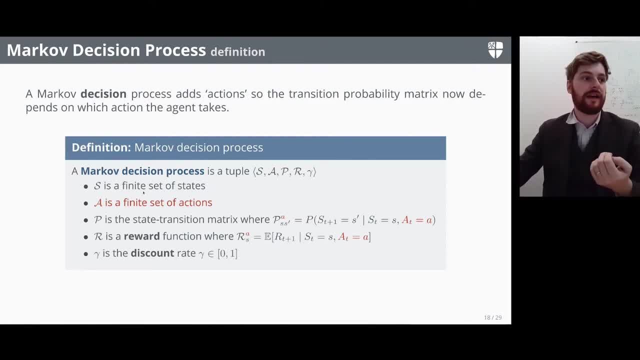 matrix for each action that you take. so we're introducing this notion of actions, so we now have a finite set of actions and it's really like saying: for every action that you can take, you have this new transition probability matrix. okay, so if we just go through here now, we have the probability for an action of 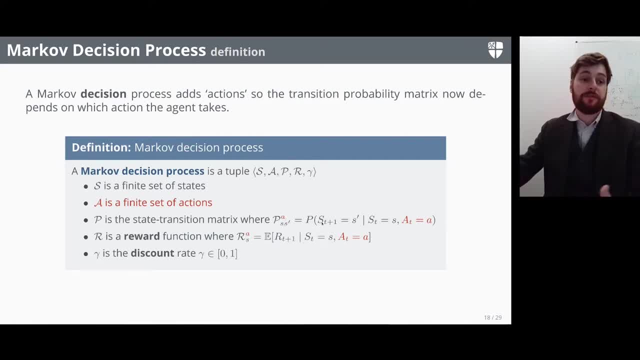 transitioning between the states. So we say it's equivalent to the probability of transitioning to the next state, conditional on a state, but also conditional on an action, And the reward function similarly we have for actions. So the reward for an action, taking an action under a state, is equal to the expected. 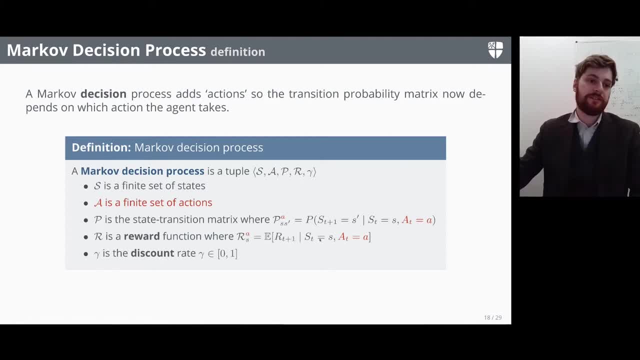 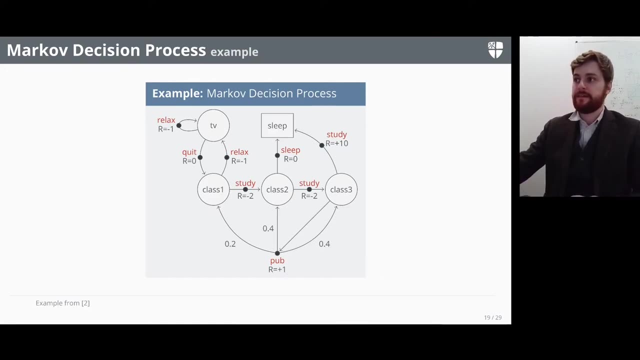 immediate reward, the expected value of the reward, conditional on being in a state and taking an action. So we add actions to our MDP and, kind of redoing David Silver's example, we now have like new decisions that we can take at any point. 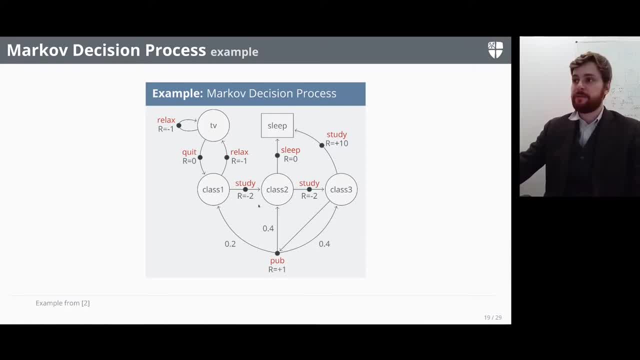 So the actions in this case are represented by black dots and they're kind of like the choices the agent can take And there's no probabilities anymore here, there's just choices. Okay, so the agent in class one can choose the action now of studying or 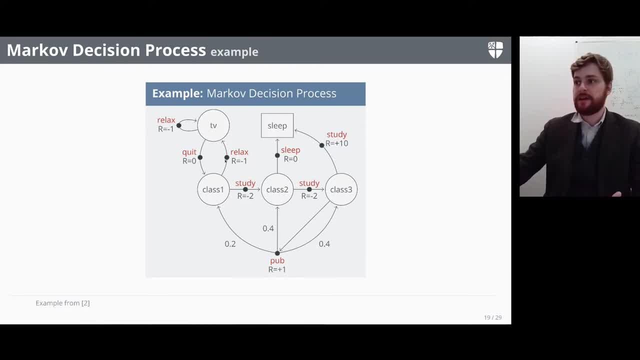 they can choose the action of relaxing, And if the agent chooses to relax, they end up in this state watching TV. But if they choose to study, then they end up in the next class, Whereas when you're in class three the agent could choose, for example, the probability via its policy of going to the pub. 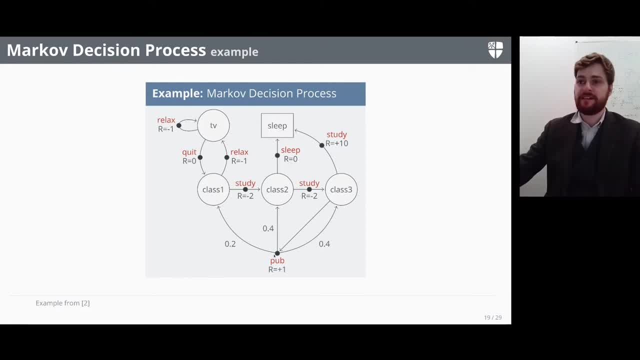 And then we would say that here is the only place where there's like some stochasticity of the action. All of the other actions are basically like having probability one. But who knows what happens at the pub? You may end up like drinking more and ending up in like one of the classes. 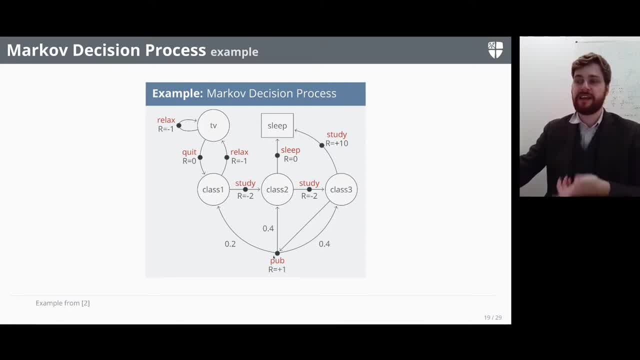 So the environment dynamics basically determines which state you end up in, So with like a Markov decision process, now the agent has a lot more control over its actions and to formalize this new control we need to define like the distribution over the actions. That's what we're going to come on to. okay. 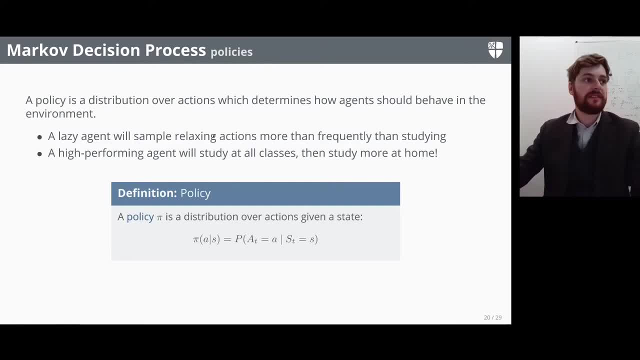 So this is really what a policy is. A policy is a distribution over the actions which determines how agents should behave in the environment, So the distributions over the actions, or actions given the states. So, in other words, if you're in some state S. 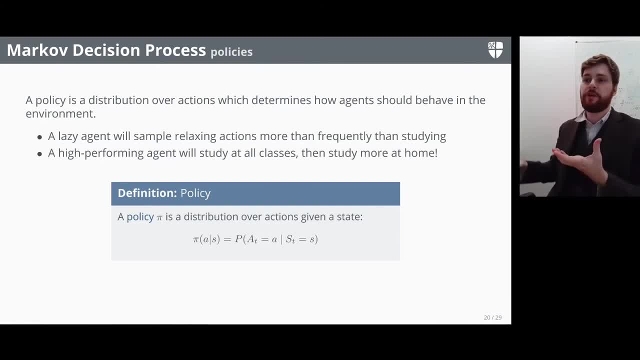 then the agent can learn a distribution over which actions it should take. if it was the class one, you could map to some probability of relaxing and some probability of studying, and you know if it's a lazy agent, if the policy is to be lazy, then it would have a higher probability. 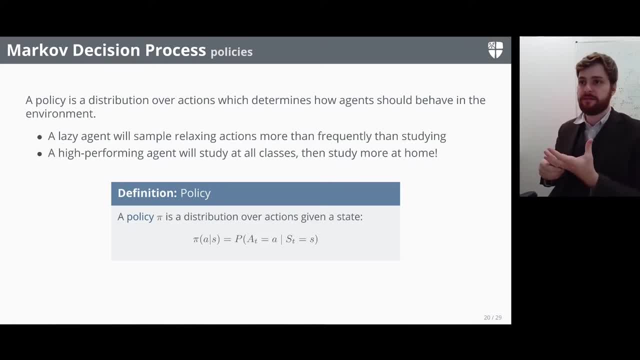 of relaxing, whereas if it's a hard-working agent, then it's going to have a higher probability of studying. So under the hood you can express that as a stochastic transition matrix, or it could be a function we learn, such as like a neural network or something. Okay, so just reading the definition, 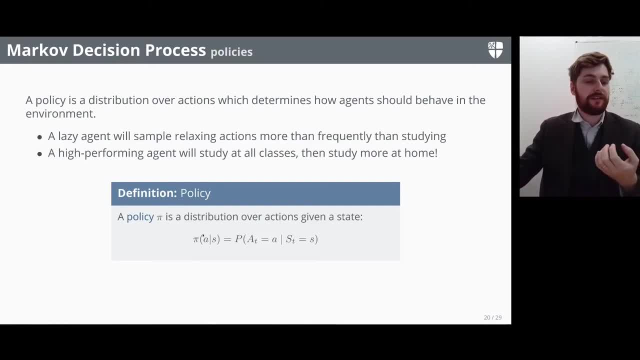 here a policy is a distribution over actions given a state, so it's this probability of the actions conditional on the state. So you may be asking yourself like: why is there no reward in the definition? and the reason is we don't really care about any of the previously accumulated reward. 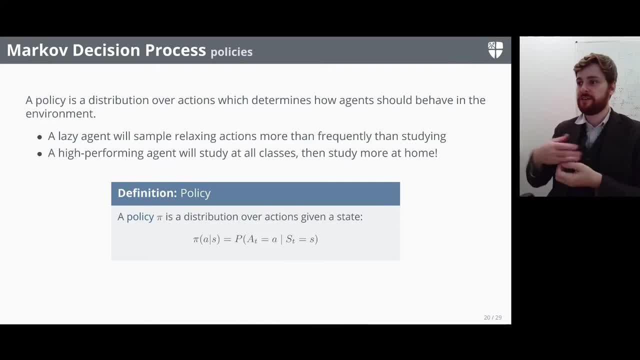 we just wish to learn how to maximize our rewards going on into the future. So if you've got like lots of money, we only care about making more money. So to behave optimally, we only care about maximizing the reward from now onwards which is captured in the future states due to the Markov property. 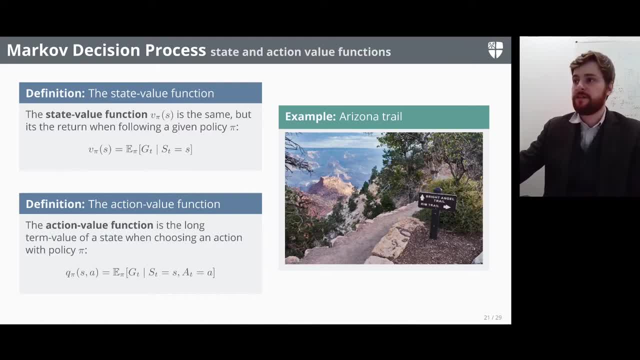 That brings us on to the state value function. So the state value function is the same. you know, it's the value function but it's not the state value function. So the state value function is the state value function, but now it's for a given policy And if you record a value function, it. 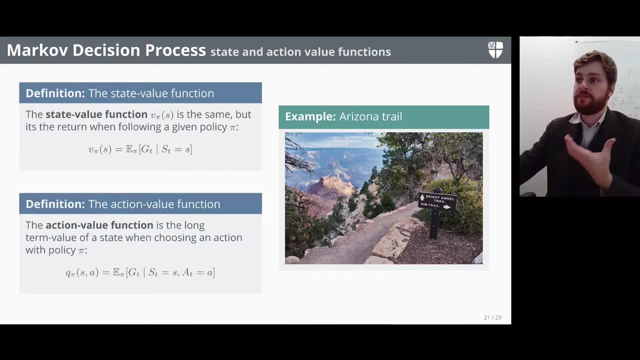 assesses how good it is to be in a given state, and it was computed by calculating the return of total future rewards. Well, now it's the same, but it depends on the policy. So again, if we're lazy we're going to get less reward than if we study hard. Or suppose, like suppose, we're the agent and 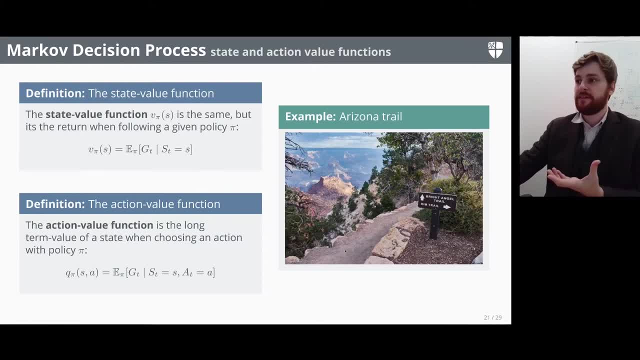 we're in a state near this bright angel trail in Arizona. There's this really nice view up in the head. So this state has quite a good value right And an energetic policy would preference skews the distribution, if you like, to just keep walking upwards, Whereas a lazy policy distribution is. 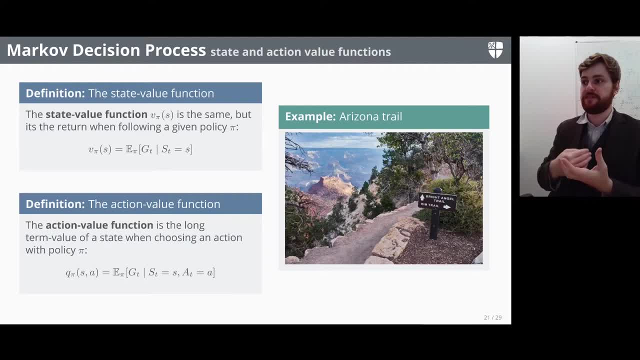 skewed to go back home And likely that policy is going to miss this S prime where it's got this more beautiful view going into the future. So that's the state value function, But also we have equally a state value function. So if you look at the state value function, we have a state value. 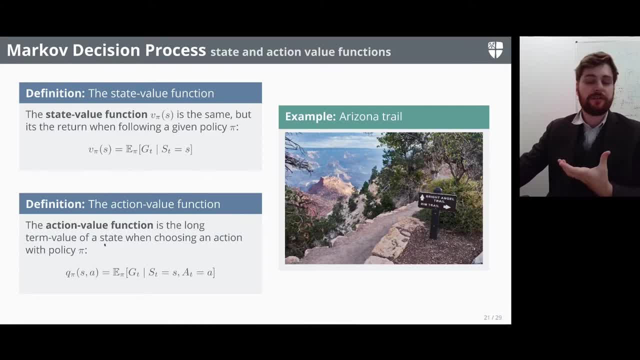 function and an action value function. And the action value function is the long term value of a state when choosing an action with a policy pi. So, for example, for my state of the on the Arizona Trail, Suppose I have two actions available. I could either keep walking and you could reach. 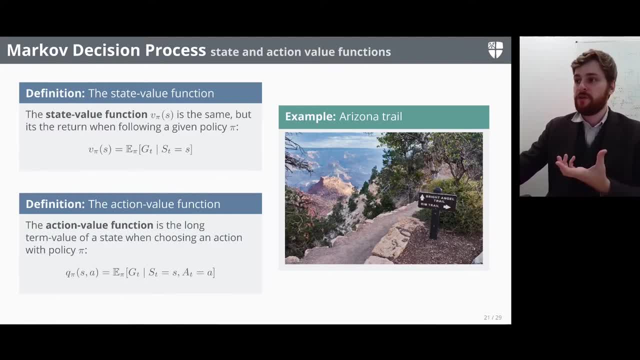 that state of having a beautiful view. Or I could choose, like the next state value function And I could choose like the next state to be to just like jump off and die. So you can see, if I was to choose the action- jump off the trail- Even if I was like following the energetic policy, it would. 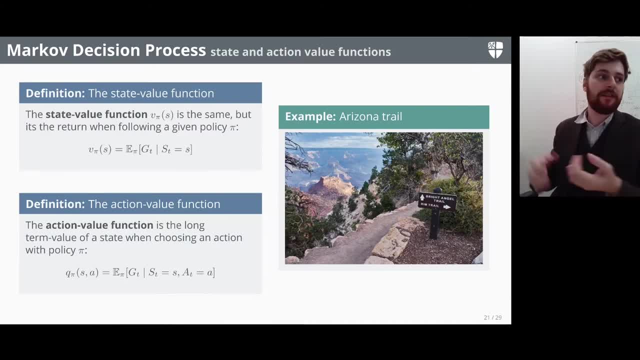 still have a very, very bad reward in the future because you'd be dead, All right. So the the action value function basically says: if I, if I'm in this state and I take this action, what is my expected return going to be under that policy If I, if I'm in that state and I've decided that I'm going to? 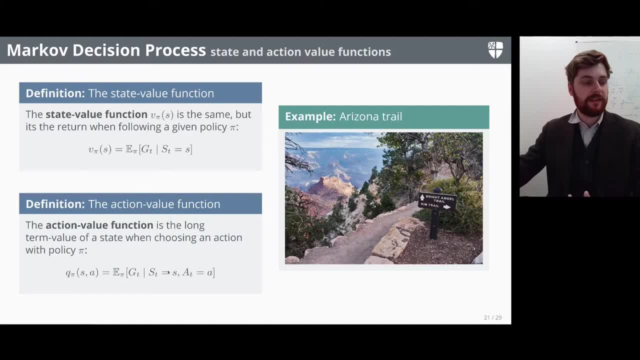 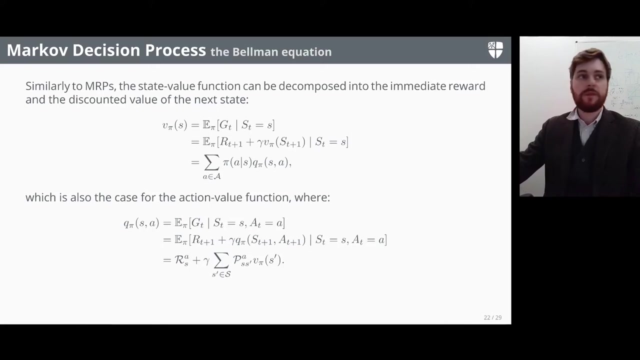 take that action All right. So it's like a- it's a little bit more information, I suppose- to the value function. It also tells us the value function If we're taking a given action, where we're going to end up. always under that policy And similar to Markov reward processes, we have the 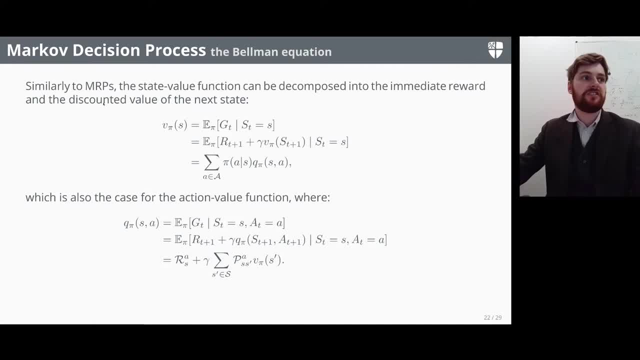 state value function can be decomposed into the immediate reward and the discounted value of the next state value function. So if I'm in this state and I've decided that I'm going to take that action over to the next state, So we can apply our Bellman equations to this. So just reading the slide, we 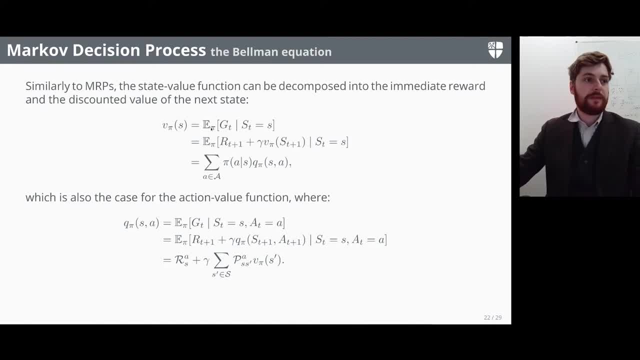 can basically say the value function is the expected return, And then we can go through all of those identities as we saw and break it down into the immediate reward plus the discounted value of the next state under that policy. And we could also similarly, as we saw. we could. 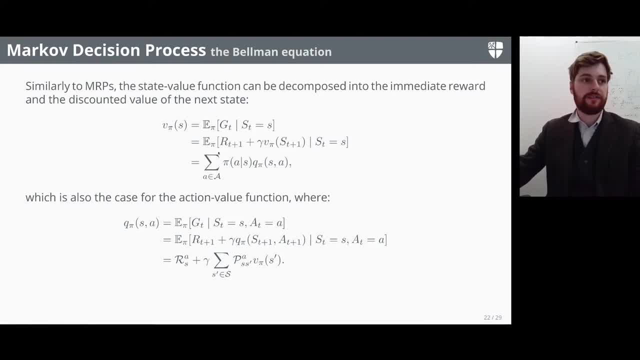 take that expectation and turn it into a summation, just by the definition of the expectation. So we're summing over the actions for the policy of the action conditional on the state times, the Q value here, which was the action value function. So we also need this. 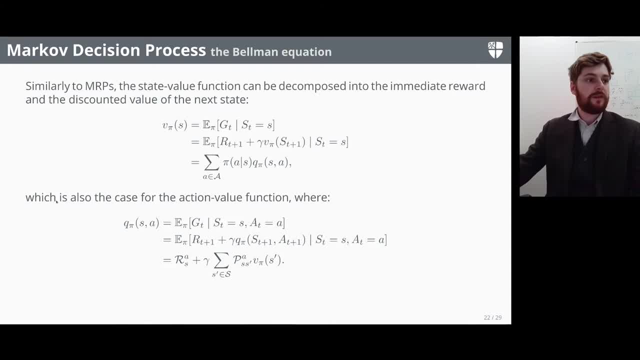 definition of the action value function which we have here. So the action value function is the expected value of the return, conditional on the state and the action which, again, we can similarly decompose. so we could like replace this action value function with a new definition. You end up. 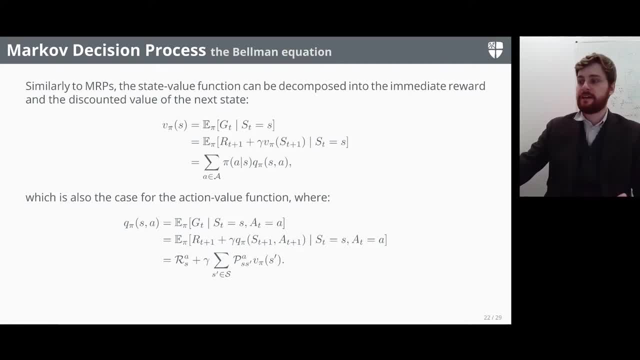 with, just like recursion, which means we can actually understand this whole thing in terms of itself, which is actually how we solve MDPs. So we could. for example, if we just look at this a bit more detailed, we have the expected value of the reward of the next state plus the discounted. 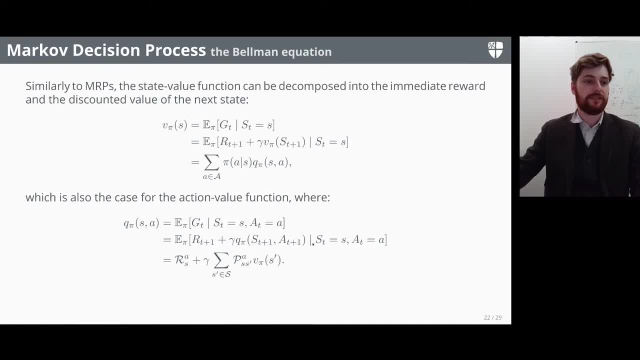 that action value function of the next state and action conditional on a state and action which, similarly we can see is the same kind of idea, it happens. It's the immediate reward for that action in that state plus the discounted value summing over all of the next states of the. 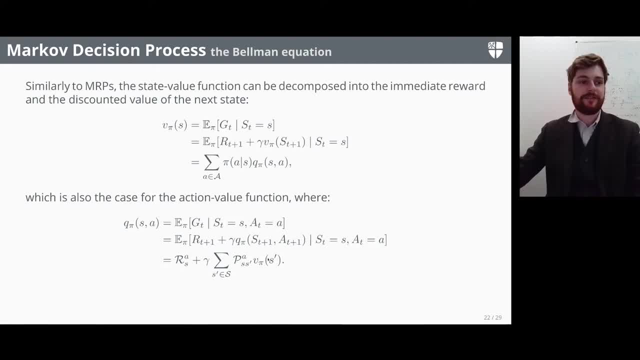 transition probability times the value function of the next state. But basically you see this value function in here. They depend on themselves. so this depends on this value function definition which itself has this Q function definition which we could take this definition for. So there's this like recursion. sorry, there's this kind of idea of this recursion here. 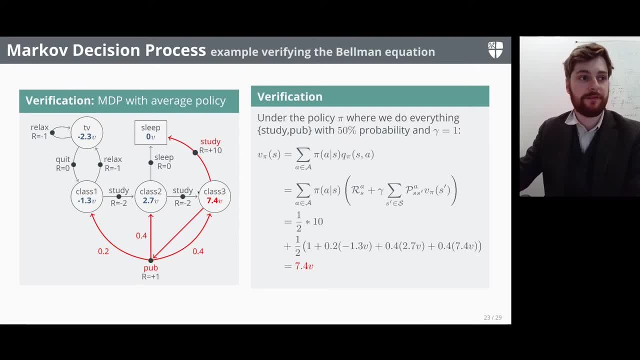 All right. so here's an example of applying that to David David Silver's lecture, where we're going to compute the, or verify that we can actually compute the very the value function for this Markov decision process. So we're going to just assume that we have some average. 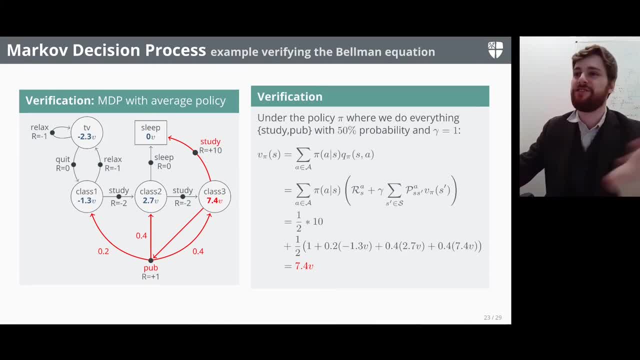 values for this, this okay. So, for example, if we have something like this here, so we would now pick this equation and we're just going to give it a number and give it a number of values, and we're just going to give it an average value function. So what we're going to do is we're 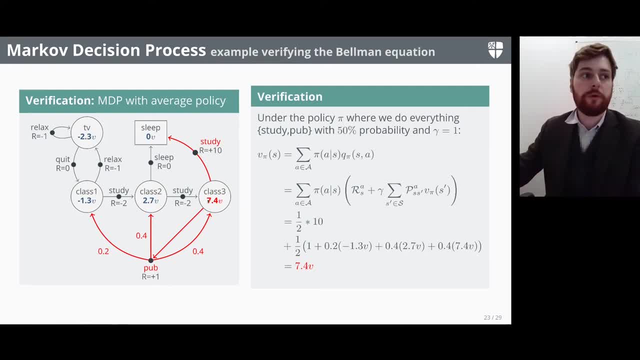 going to take all of our values and assign them here, but we're going to do something like this. So we're going to take that 16 and we're just going to add that over here and then we're going to take for value here. 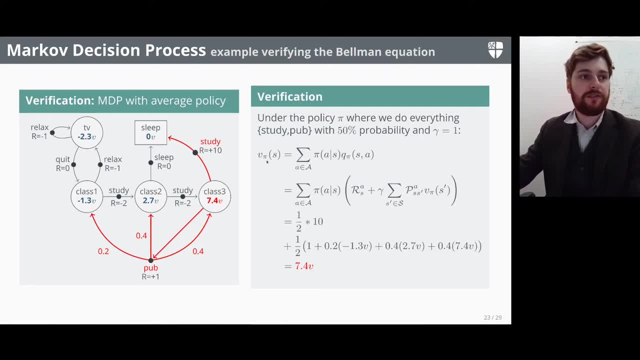 And I'm just going to show it by verification. So the definition of the value function being in that state under that policy is as we just had in the previous slide, And what we tend to do is we reach this Q star and we just take the definition of Q star. 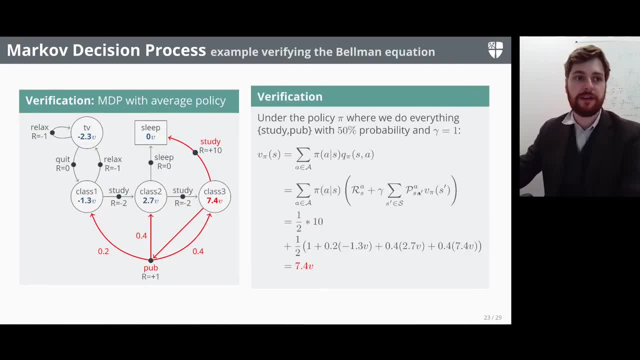 which is here, and we substitute it, So we now have just this larger value. This is what we're going to use this equation here. So, actually applying this, what it tends to do is it's like a one step look ahead. That's the best way to think of it. 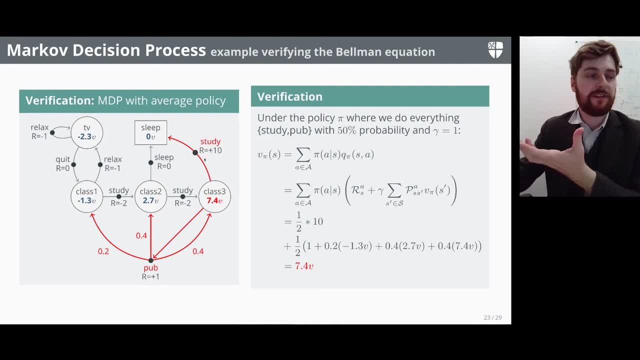 All right, so let's just start by this action here. So there's 50% chance under this policy pi of taking this action. So it's 0.5 probability. So this is the policy, So it's 0.5 probability. 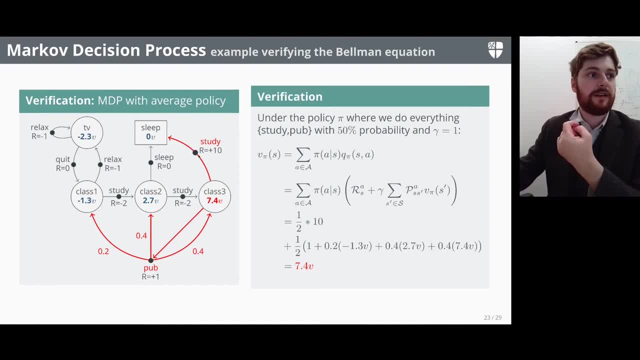 So one over two here times the reward here plus, and there's nothing in the future for it to consider. So this all just zeroes out. So we just get 0.5 times 10 for this action here. Okay, but then we add the value of being in this state. 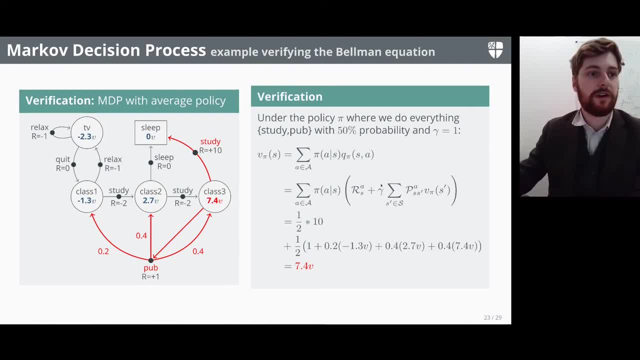 of taking this action here, which is a little bit more complicated, So let's just work our way through this. So we have 0.5% probability under our policy of going to the pub. So it's 0.5 for us. 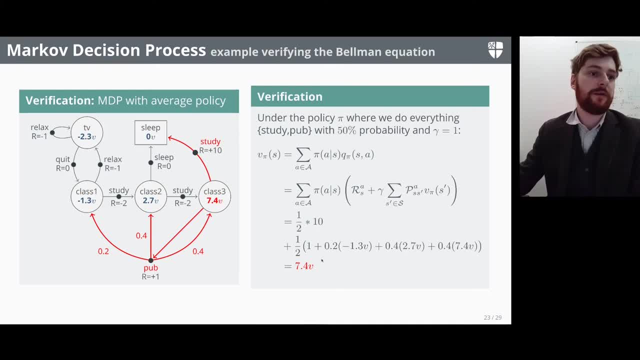 So that's our policy. pi here times, And now we're gonna do our one step. look ahead, So this is all of this stuff here, So it's the immediate reward of being in the pub, which is simply one, And then what we do is we add our discounting factor. 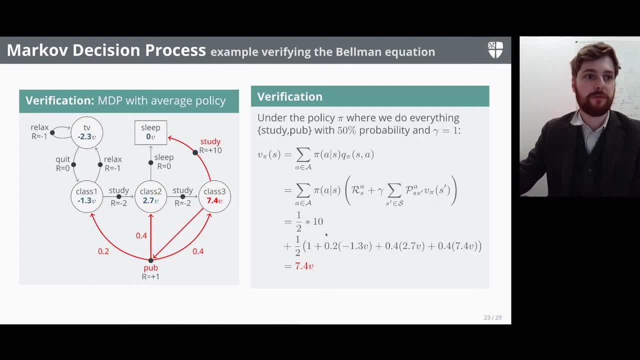 and we said that's one times, So we can just get rid of that one cause. it's one times something. And then we're going to be looking at the future states, value functions And they're probably at times, by their state, transitional probabilities. 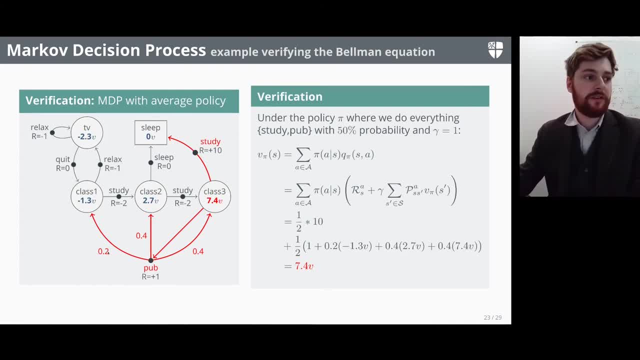 So when we're in the pub, the next state is gonna be class one. So at 0.2 times negative 1.3, the value of negative 1.3 plus 0.4 probability of going back to class two. 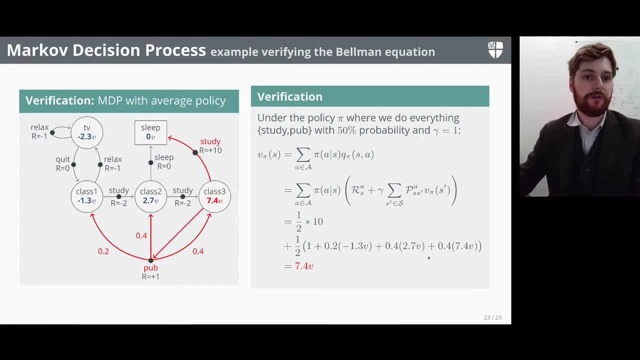 which has a value of 2.7, plus 0.4 times the value of going back to class three, which is 7.4.. And then when you add all of that together, so you've done this kind of one step, look ahead. 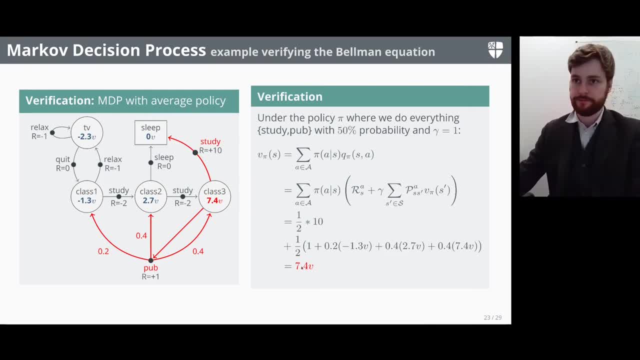 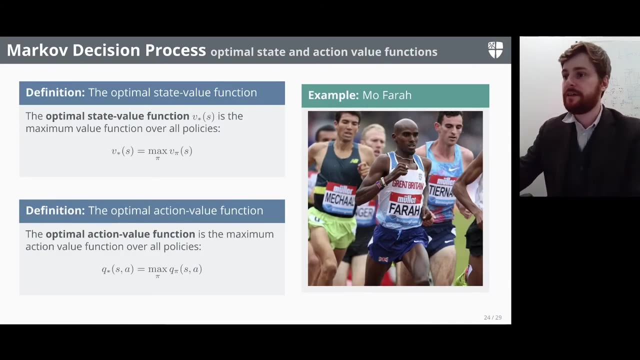 process you get the final value, which is 7.4.. So that verifies how we can use the Bellman equation with that kind of one step. look ahead, local bit of computation to compute the value function And, yeah, you can actually solve that. 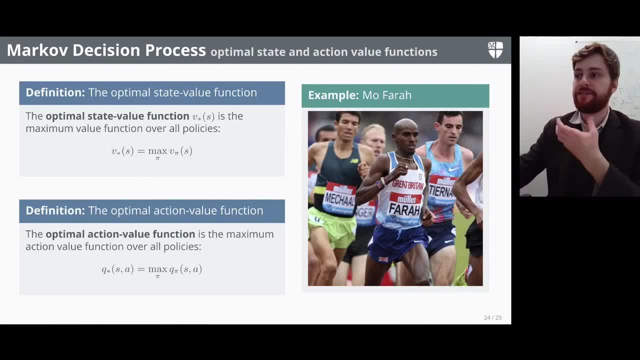 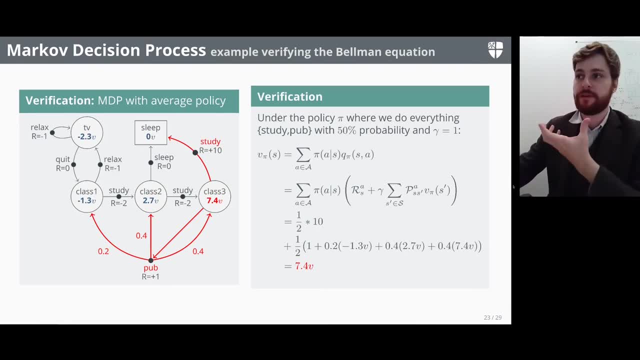 for a given policy directly again achieved by averaging it. So sorry. So you could end up with like a Mark of Reward processes which was solvable as a linear equation for that given policy, And it's all very well. 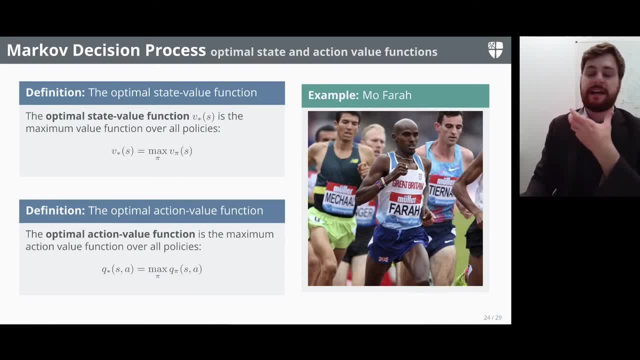 because it tells us like the expected behavior, but it doesn't really tell us how to behave optimally. All right, What we really care about is figuring out how to optimally play these games, So, for example, like Mo Farah, winning the gold medal here. 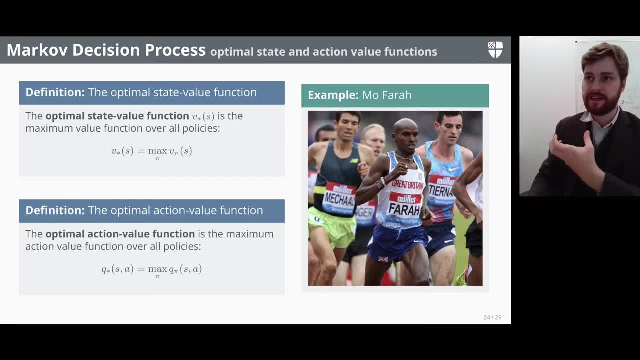 for him to get the best possible value, he must also have the best possible policy, which is like doing all his warmup routines, his dieting, his pacing strategies. And if we let's just read the definition of this, which is to say that the optimal state value function, 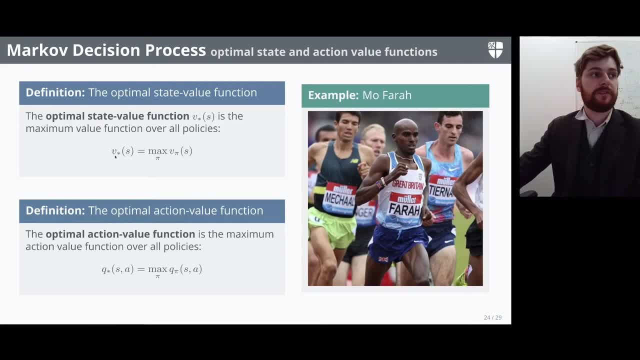 is the maximum value over all policies. So the optimal value function for being in a state is the maximum for all policies, the value function of being in that state And V star here tells us the maximum amount of reward you could extract from the system. 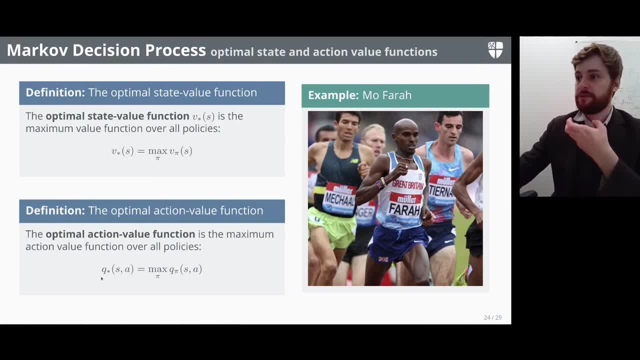 So, similarly, Q star or the action, the optimal action value function tells us the maximum amount of reward you can extract when you start in that state and you take that action A. So what's the best time Mo Farah could possibly get if he chose to eat a hamburger? 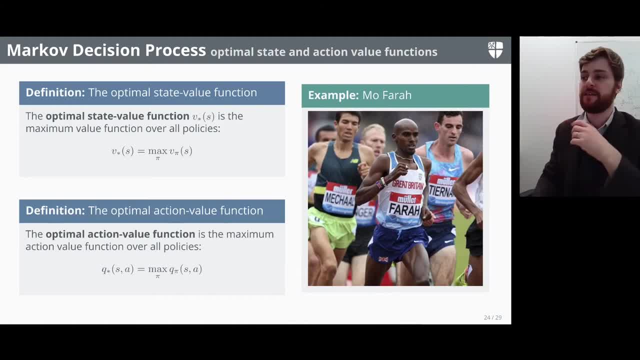 instead of his usual chicken and rice in the morning of the race. But then if he did everything optimally from there on all his training and his warmup routines and his pacing, if he did that all perfectly, he would be able to fix the game. So, for instance, if he did all these things from there on all his training and his warmup routines and his pacing, if he did it all perfectly, If he did it all perfectly, 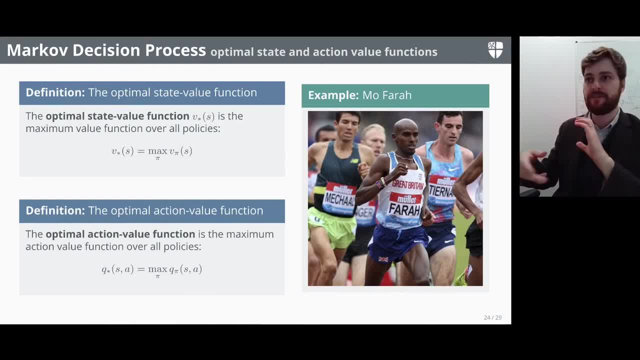 What's the maximum time or the best time, I suppose the smallest time he could possibly get, And if you have Q star, you're done. The MDP is considered solved because it tells us everything we need to know to behave completely optimally from there on. 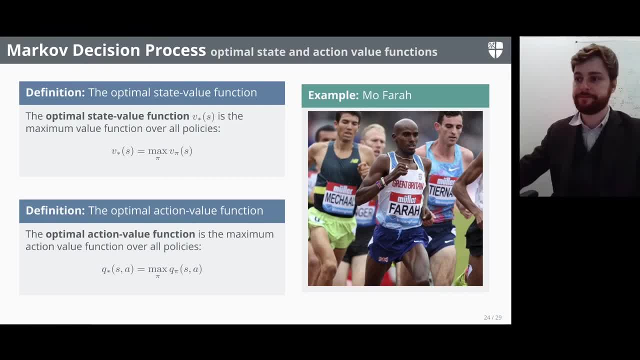 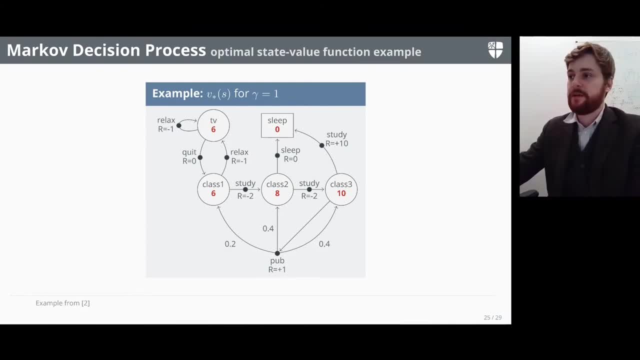 It tells us which actions to take at which dates to always win. So we can kind of just eyeball this to see how it works. So like, if you look at this example here of these optimal value functions, if you're in class three here, should you go to the pub or should you study? 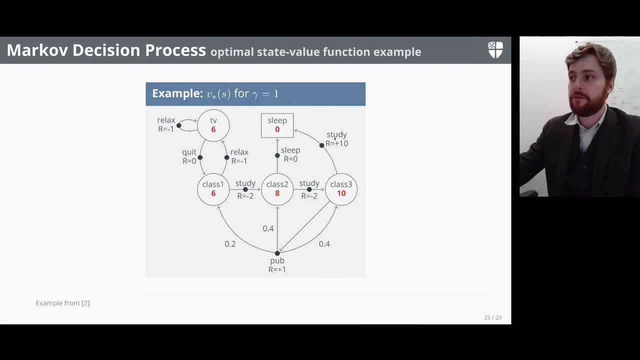 Well, 10 is the optimal value. That's where we get our reward. So the max of 10 and 1 is 10.. So you should study. That's the best action you can take in class three is clearly to study. 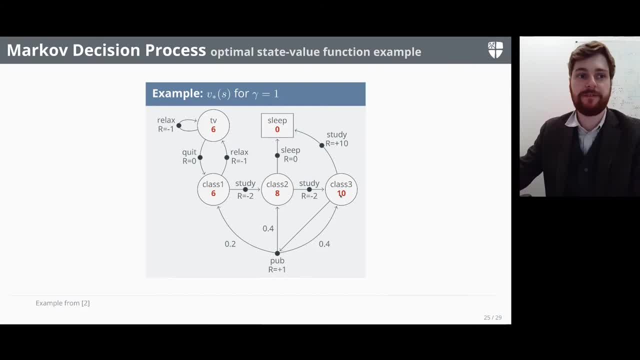 And if we kind of back up now with that value function, that optimal value function, and look at class two, then we can either choose to sleep with a value of zero or we can study and get a nice juicy value of 10.. 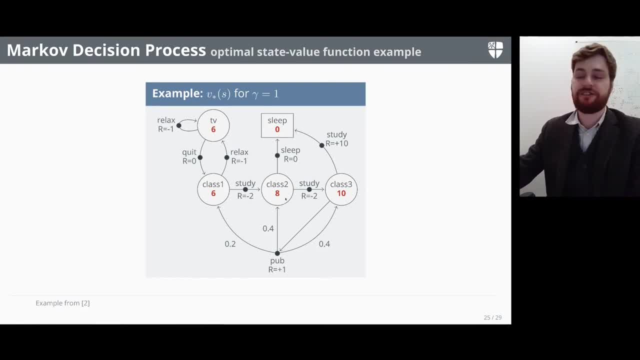 But we get minus two along the way. So the value is actually eight. And back up now to class one. we could again. we again would lose two rewards. So the optimal value is six. And lastly, the TV state. we can either choose to lose reward by continuing watching TV or we can quit at no loss of reward and return to six. 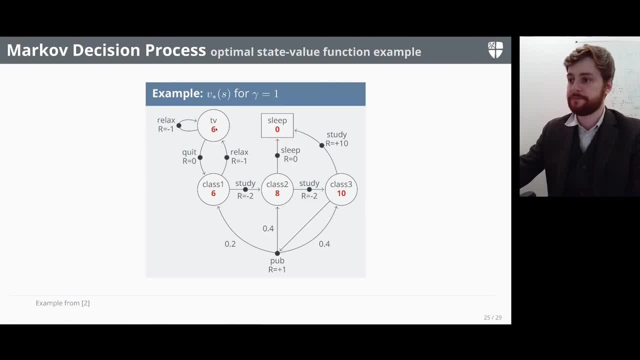 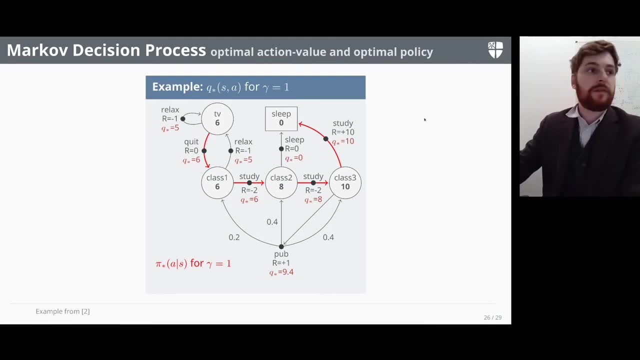 So there's no loss of reward here. So the optimal value is six. Okay, So we can kind of just see that intuitively. But we also have, like the optimal action value function, Q star, And this similarly tells us which action. 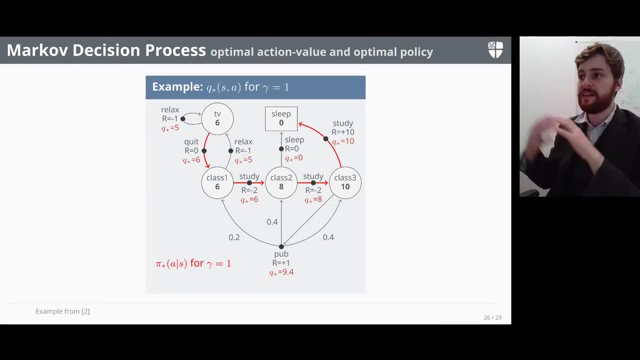 We must take to always win. So in other words, it weighs, it weights the edges and we can just follow the edge with the highest value to always win. So if we notice we're done, for example at class one, here we can see that the action to relax has a an action, an optimal action value function of five, and the action to study has an optimal value function of six. 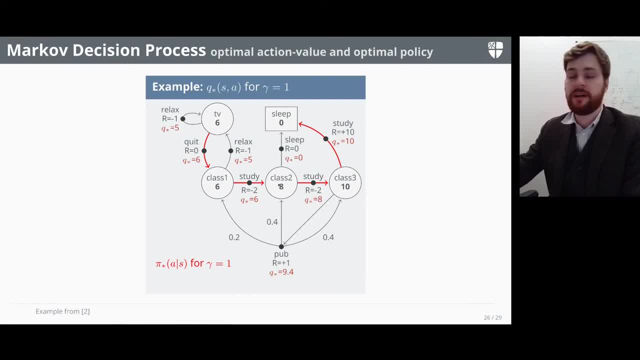 So so we study, we always just choose the max, And if we're in class two, then we can see that the action to sleep has a Q star value of zero and the action to study has a Q star value of eight. 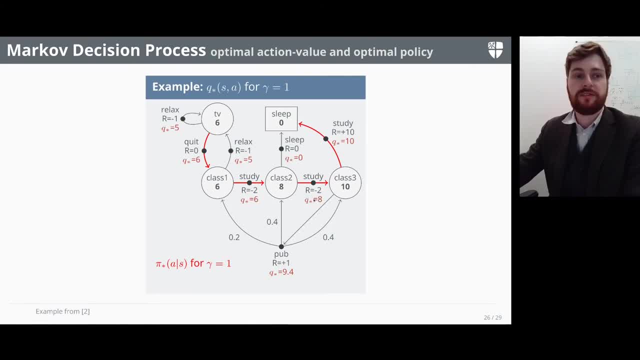 So we we always take the max, So we always study again here. And if we're in class three we can see the action to study is 10, and the action to go back to the pub is 9.4.. So the max of 10 and 9.4 is 10.. 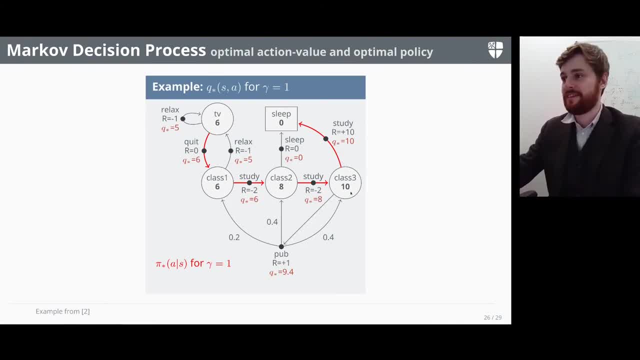 So we, we would study here. So it's, it's reassuring to see that the optimal strategy Is to indeed study. uh, yes, it's better than going to the pub. Um, so we'll see how to actually compute these optimal value functions. but the optimal policy is therefore shown here in the red edges. 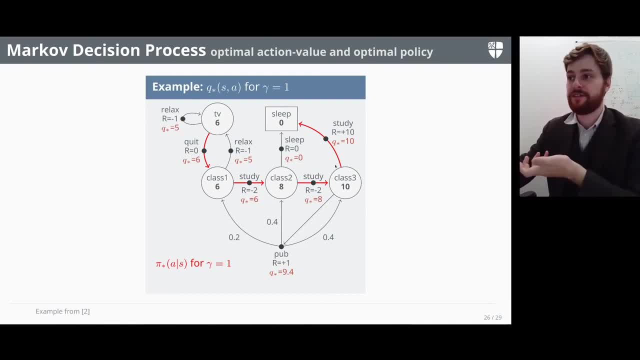 Okay, And it intuitively relates to the optimal action value function. The optimal policy is always the one that picks the highest Q. Okay, So we can see that the optimal policy- and that's for gamma- is equal to one. So how do we actually 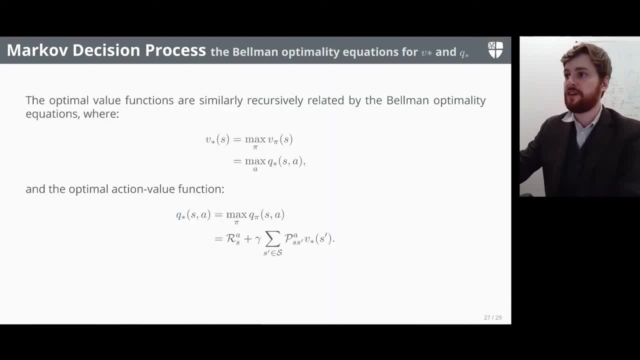 Compute that central quality, uh Q star, while we do what's called the Bellman optimality equations and we work our way backwards from the final state. So just looking at the definition here, um, they're similarly recursive, the related by the Bellman uh optimality equation. 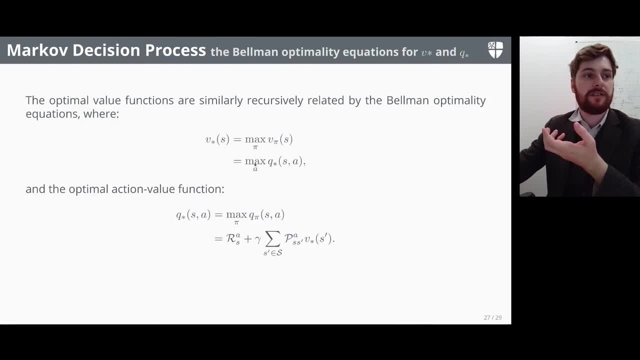 So this idea that the optimal value function is the max Q star, whereas Q star um is also relates to the Bellman expectation Uh equations which we we saw earlier. Okay, Um, so there's this kind of recursion definition, recursive definition again. 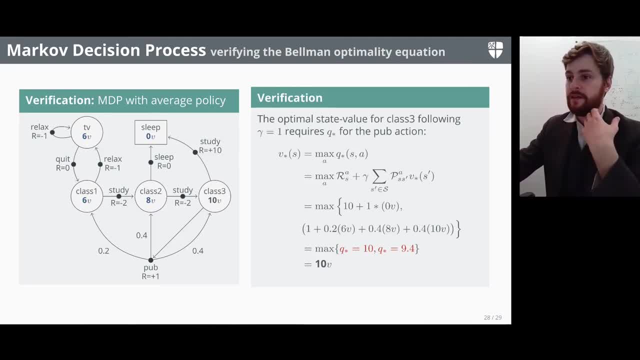 So, just to make this concrete, we'll have uh a sort of last example of how we can compute uh the value, the optimal value function and the optimal action, the optimal value and the optimal action value function, So V star and Q star. 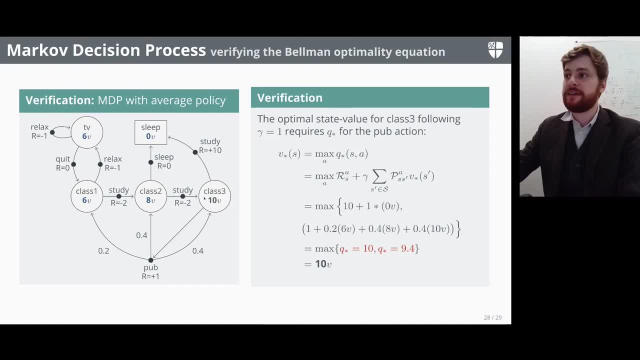 So for class three here, um, if we record a definition of V star from the previous slide, it's equal to the maximum action value function. Uh, and then we can just take that definition out: Uh, so it's the maximum of the reward for being in that action, plus the discounted something of the next states. 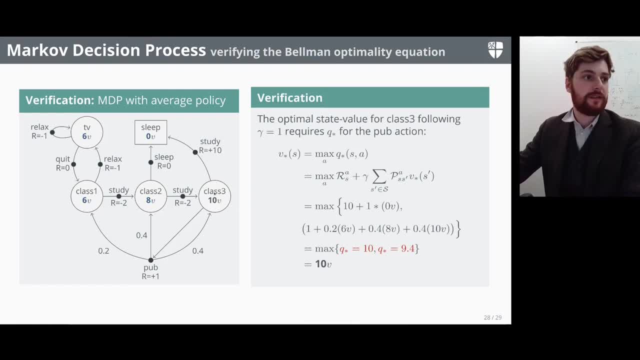 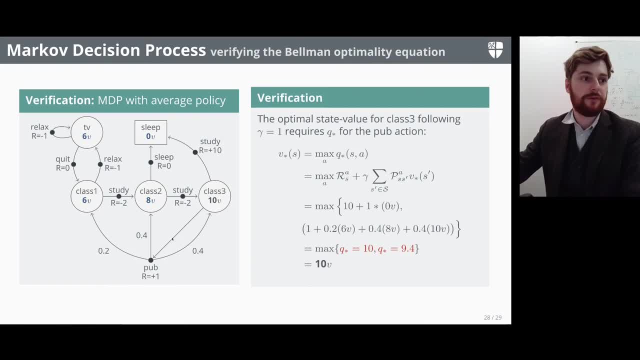 Uh, and then we've got to sort of look at it going forward. for going down here, where we've got again, it's discounted by one plus there's this: uh, 0.2 probability of getting six plus 0.4 probability of getting eight. 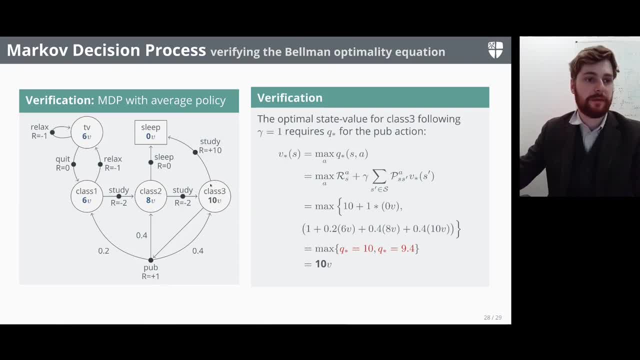 Uh, and then plus 0.4.. Uh, and then plus 0.5 probability of coming back here, Uh, and then plus 0.5 probability of coming back here, And if you sort of assembled that all together, you've now just got the maximum of this Q star being 10, and this Q star which, that all gives you 9.4, which gives us your final 10.. 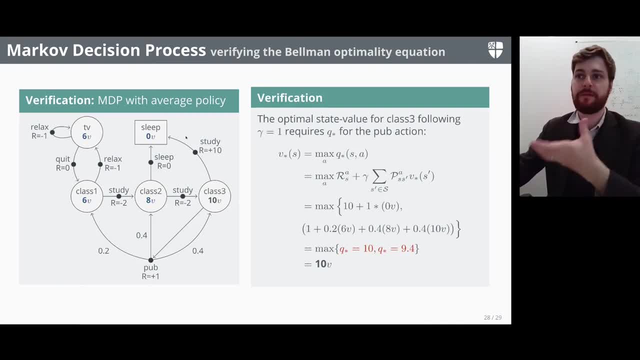 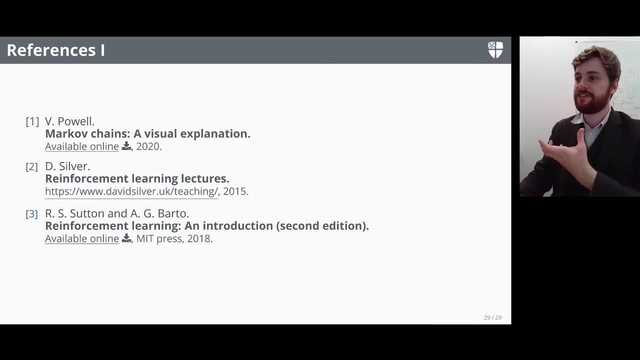 So that's how you actually compute it again, with this kind of one step look ahead idea which is very similar to the example we saw previously. So that kind of concludes this lecture. Um, I appreciate there's been quite a lot of maths and formal notation, uh, which does take a bit of time to sink in.